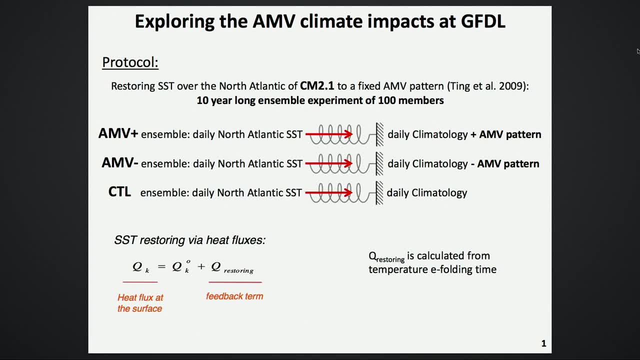 So CM2.1, it's a one degree oceanic resolution on a 200 kilometer atmospheric resolution. And so we can see that the CM2.1 is a one degree oceanic resolution on a 200 kilometer atmospheric resolution. Okay, 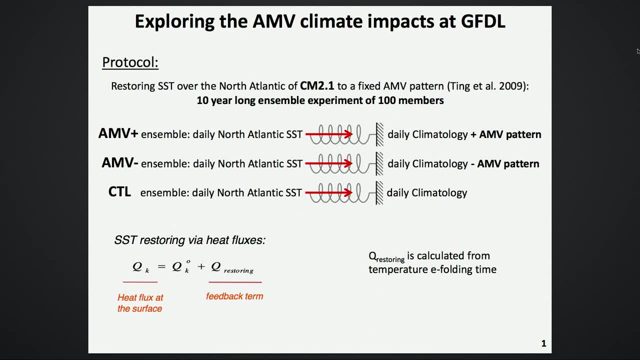 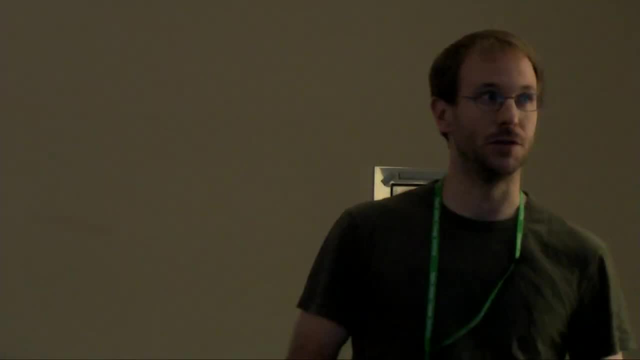 So we restored the SST over the North Atlantic to the fixed IMV pattern as defined by Tigetal 2009.. And we did a 10-year-long ensemble experiment on 101 members. so in order to estimate the signal channels of this influence, 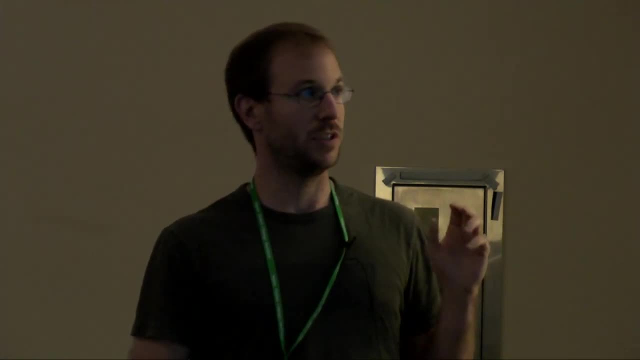 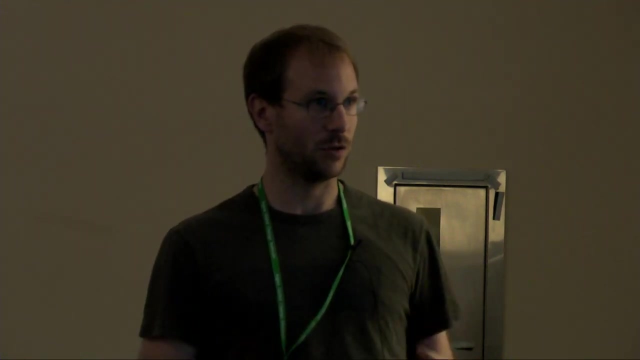 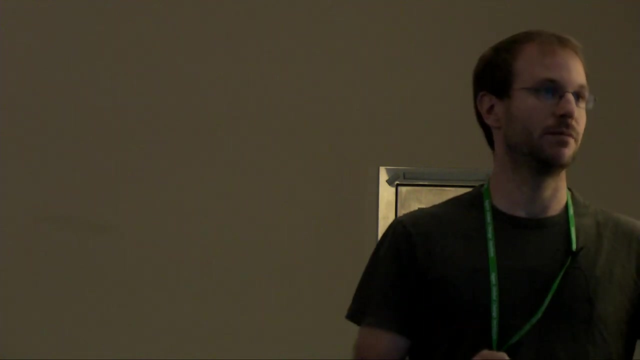 So there is basically three main simulation. The first one I call the IMV+. So we restore the North Atlantic SST to its climatology, to its deltas, And we add on top of that fixed positive SST anomalies. that is the IMV anomaly. 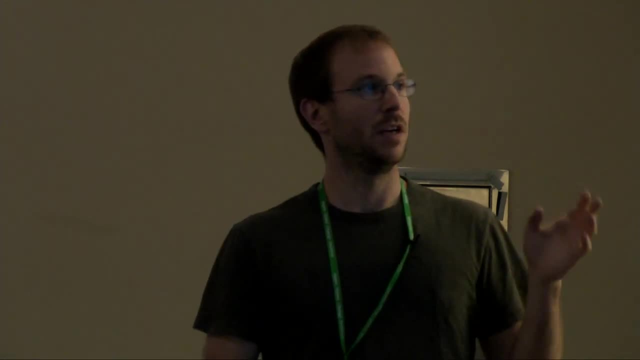 So we've got the IMV- experiment that is the same as the IMV-plus experiment, but with a shift of the sign of the IMV. And because this protocol, we expect that this protocol restoring the model to its climatology. 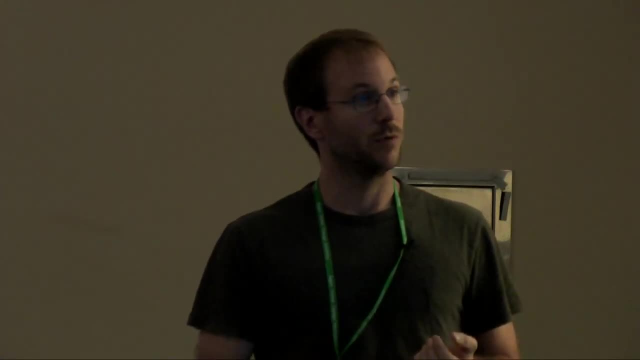 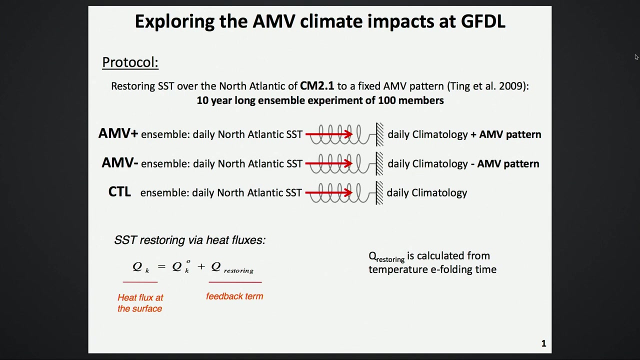 So to change a bit the main state, we did a control simulation where we just restore the model to its climatology. So the restoring is done by eight fluxes. So the restoring is done with a five-day time scale with a mixed layer depth of 10 meters. 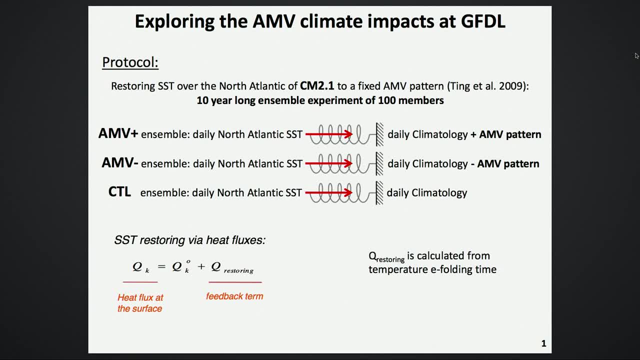 So that is equivalent to the Okay. So that is equivalent to the third case that Christophe showed yesterday, with a restoring of one-on-one on 20 watts per square per second. So it's quite soft. It's not so strong for who are still respecting the coupling, et cetera. 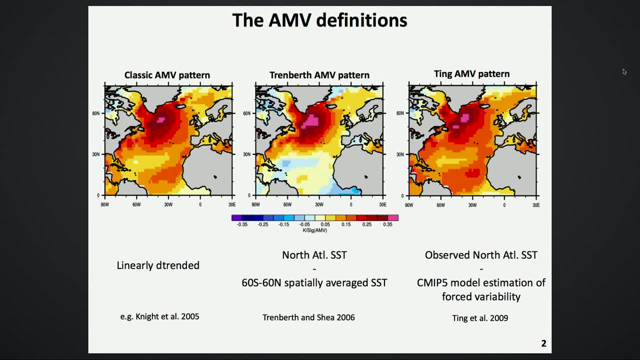 So about the IMV definition? what did you choose? So here is a different definition of the IMV, So what I call the classic IMV, the trend-based IMV and the TING-IMV pattern. So the different. 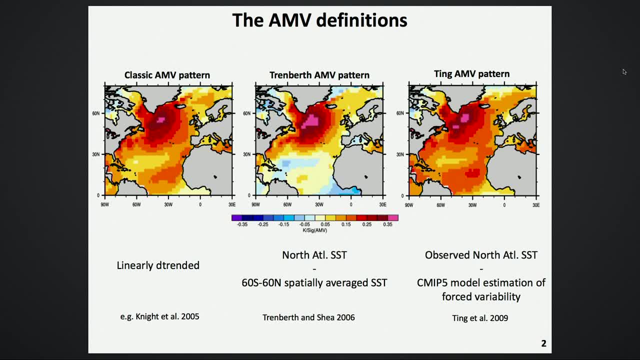 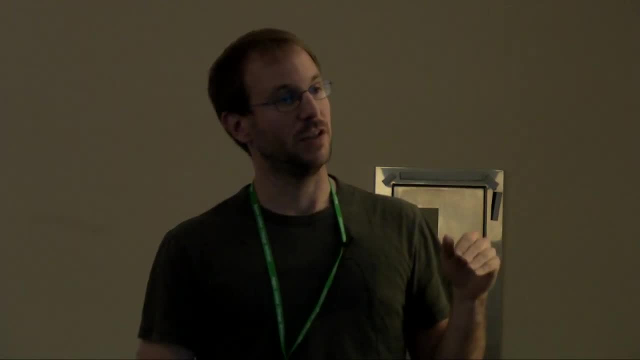 So the difference in this IMV pattern is only due to the way you remove the trend, the external forcing. So in the classic case you just remove a linear trend. In the trend-based case you remove to the North Atlantic SST the specially-averaged 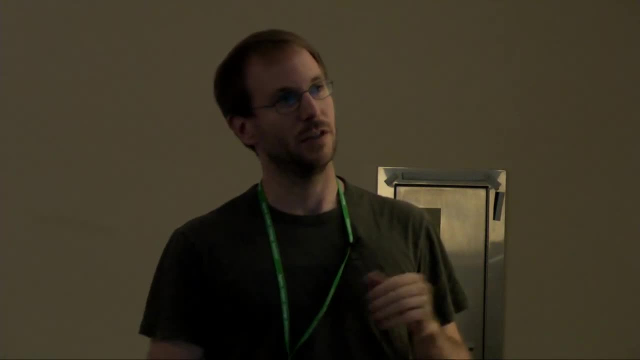 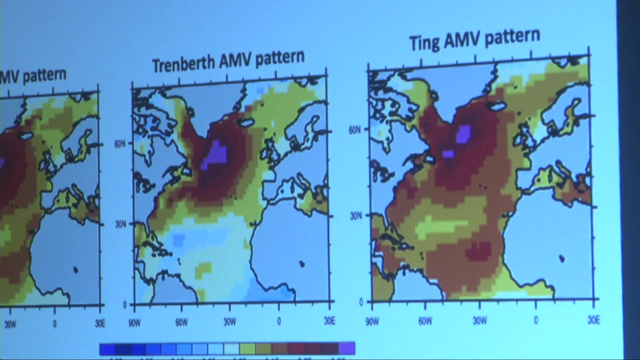 SST of the globe and in the TING-IMV as TING presented two days ago. I guess you remove the external forcing. So that's the new estimation from the SEMI-5 model. So we choose this IMV pattern because we think that it's the best estimator of the internal. 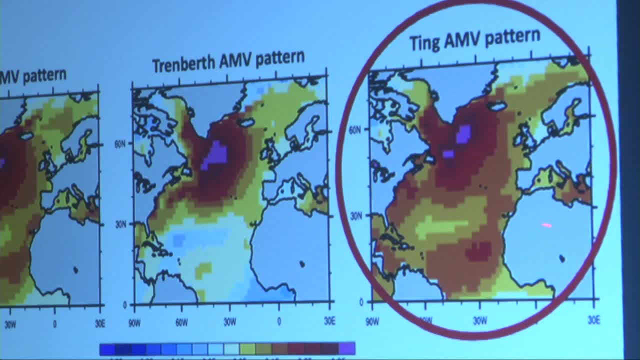 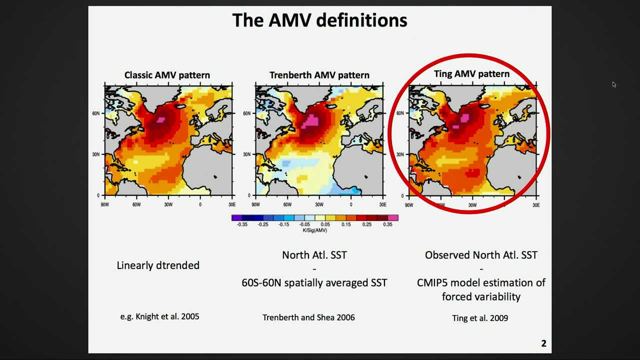 variability so far, but we have to keep in mind that there is discrepancy between the IMV pattern, the IMV definition and, especially in the tropics, between trend-based and TING-IMV, And I will show that it can lead to different IMV impact. 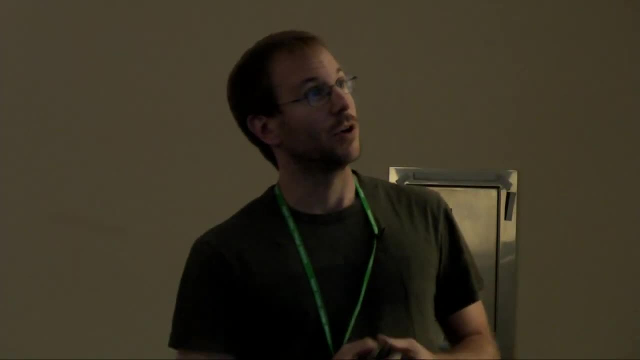 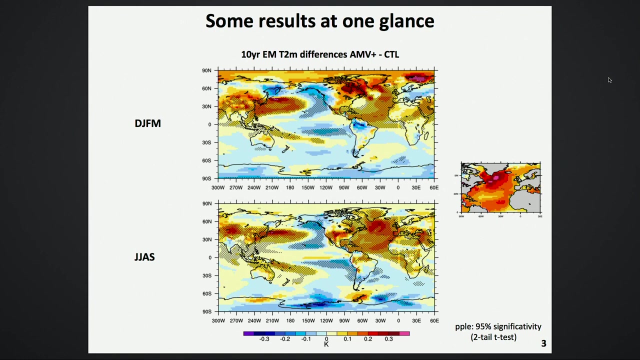 Yeah, So some results quickly. So this is the 10-year ensemble mean difference between the IMV-plus experiment and the control experiment in terms of surface temperature. So here at the top is for the season, DGFM, on bottom for DGAS, and here I recall the 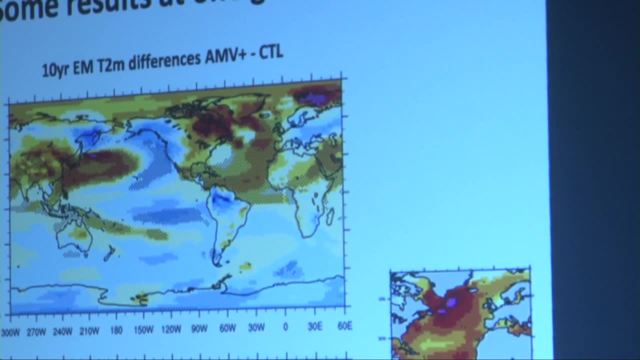 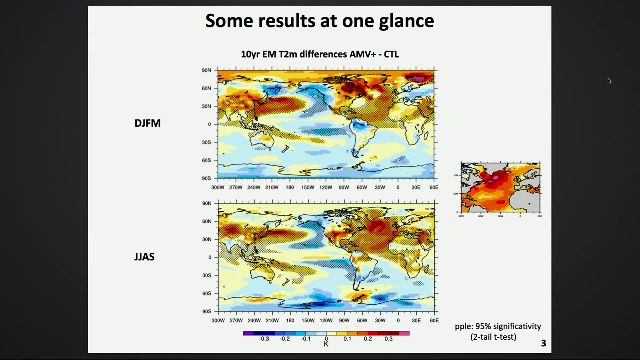 TING-IMV pattern to which we try to restore our model. So in DGAS we can see that our simulation, The simulation, do kind of a good job. It's a bit weaker, but the pattern is there and the structure is there, whereas in DGFM. 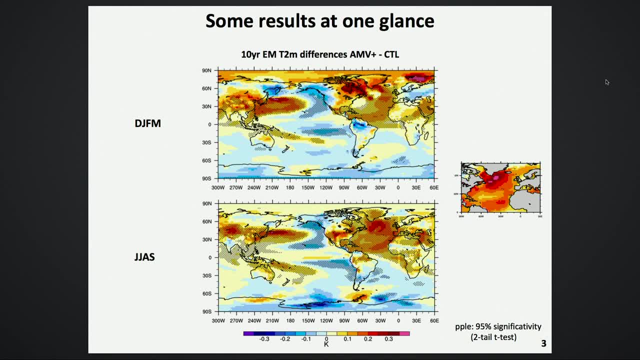 it's much more noisy and we can see that in the Labrador scene- Labrador, on a super large area region- we can see warming, and this is due to two reasons. First, in winter you increase your mixed layer depth, so it's more noisy. 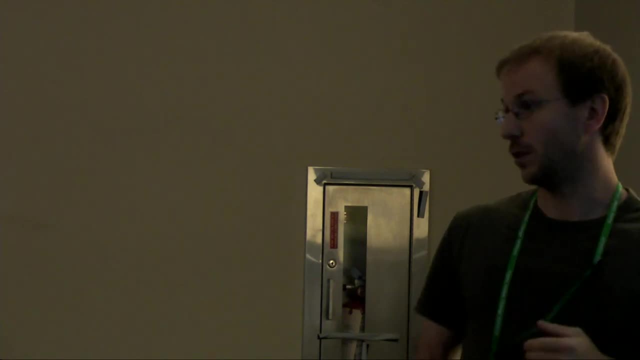 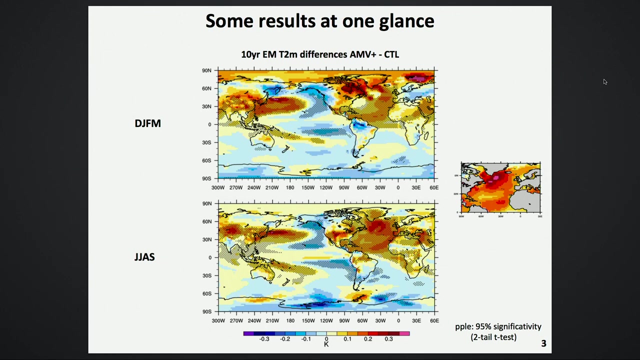 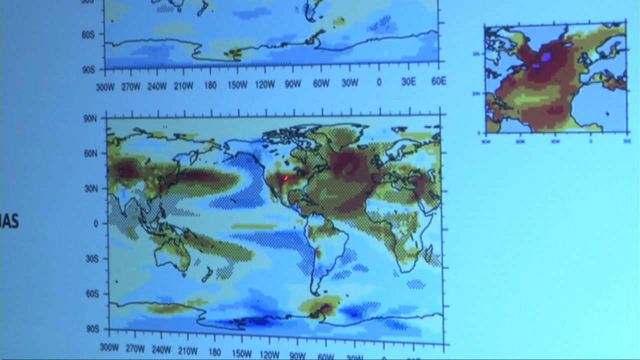 And the second reason is there is a drift in the simulation and Raymond is going to talk about that later. So if you look out of the Atlantic we can see that over land in DGAS there was a warming over a stratopical latitude over land. so over the US there, over all the Mediterranean, 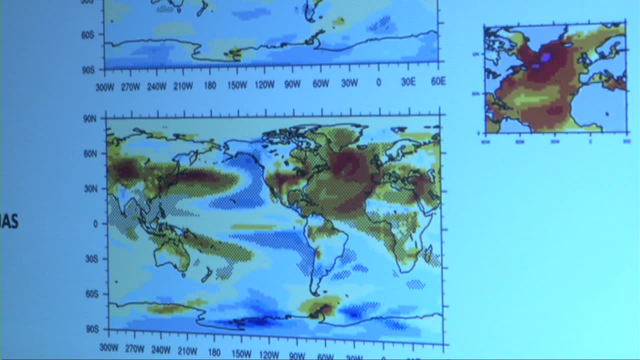 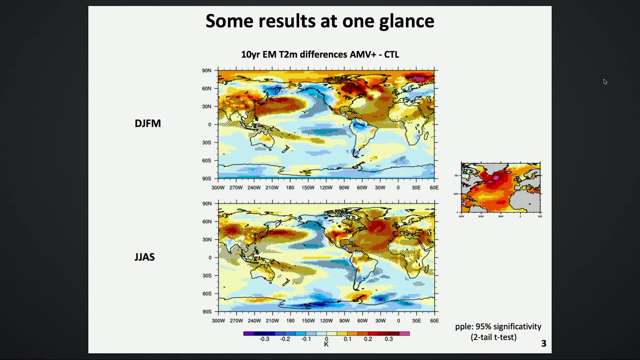 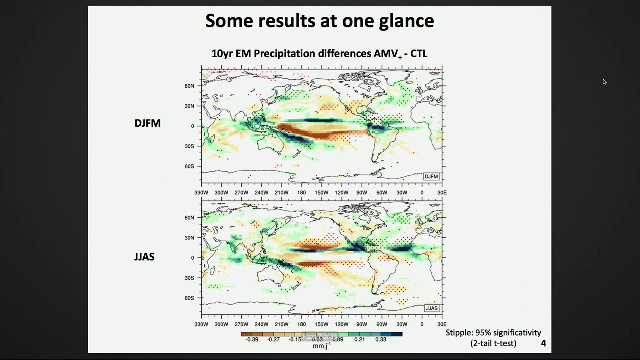 basin and over Asia. In winter there was no warming there, no warming there, nothing significant. but there was still warming over Asia there And we can see a strong PDO. Okay, The response of the Pacific here In term of precipitation. so blue means increase of precipitation and red and brown decrease. 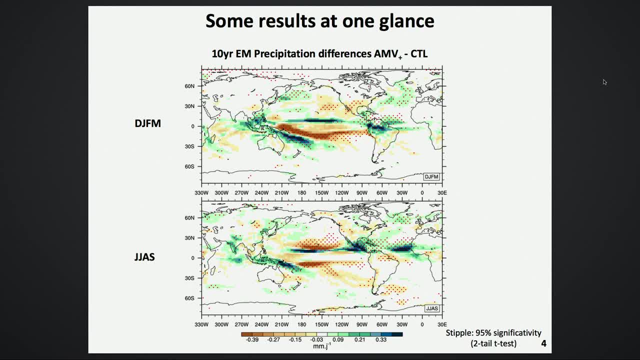 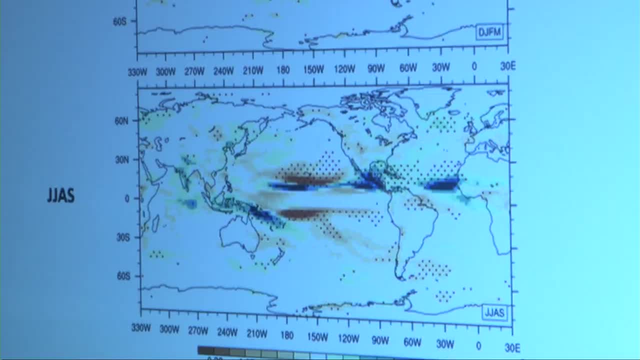 of precipitation. So we can see in DGAS an increase of the northward part of the IT state over Atlantic and as well over the eastern part of the Pacific And over the western Pacific we can see a tilt of the ice species head to the west like. 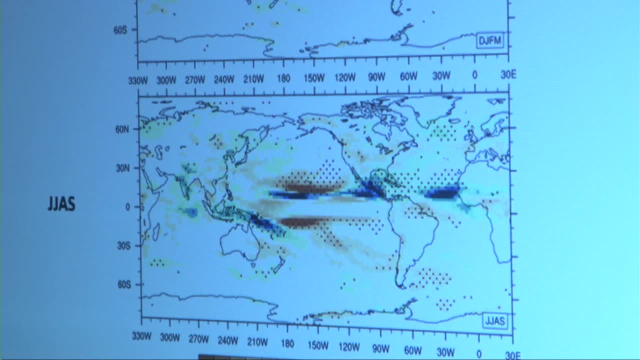 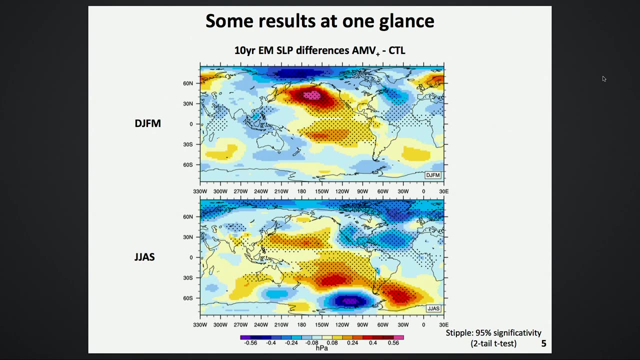 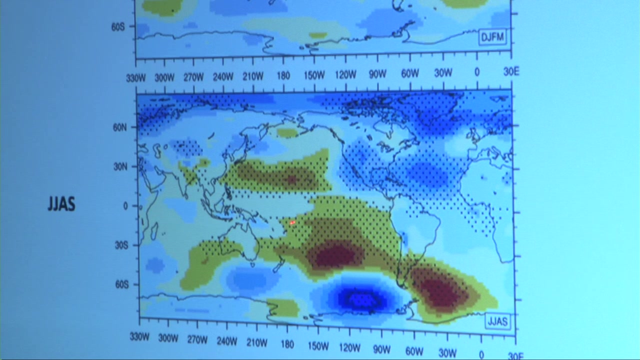 that And this is. we can see that as well in DGFM. In term of sea level pressure, in DGAS, we can see a low pressure anomaly over the entire North Atlantic that is mass compensated by high pressure over the Pacific. This is for DGAS, and we can see similar things for DGFM, even if the low pressure is weaker. 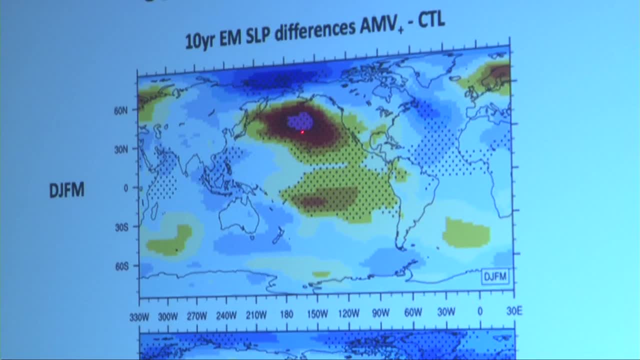 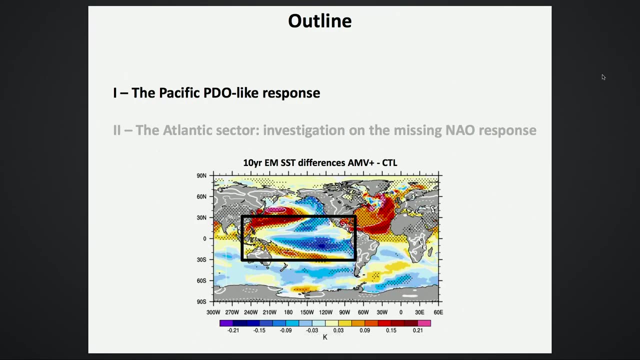 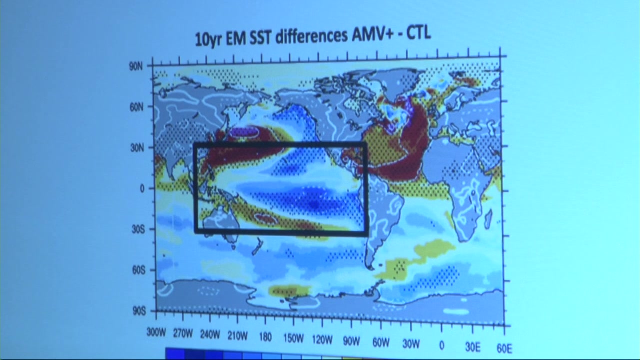 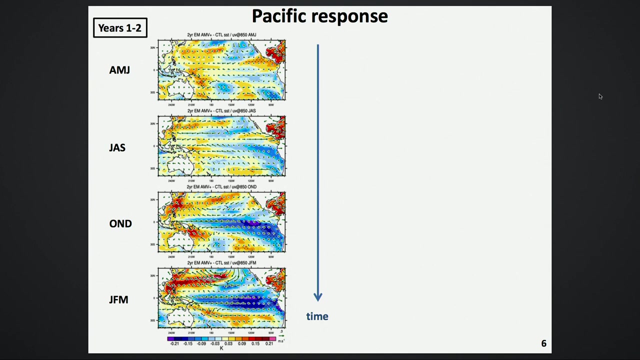 over North Atlantic And we can see a strong response over the Aleutian low here. So today I would like to mainly focus over the tropical Pacific part of the response And I am going to explain how this response happened. So to explain how it happened, I just focused for the moment on the first two years of the 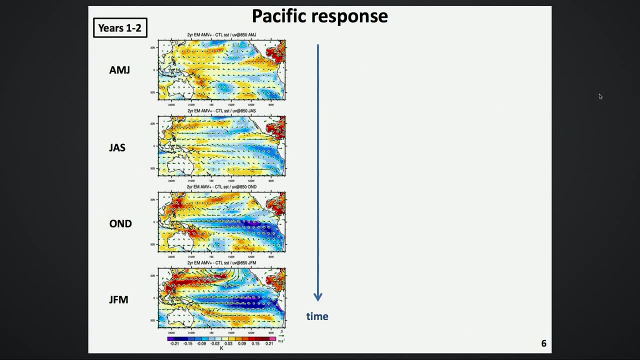 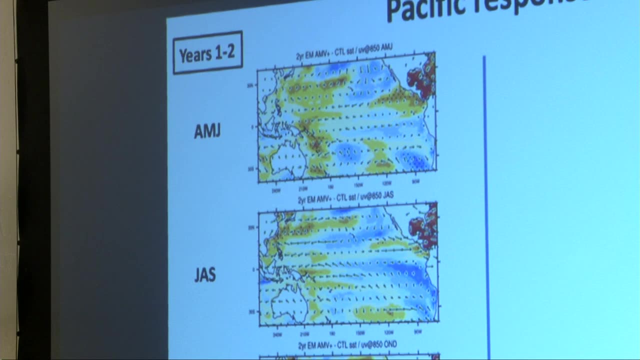 simulation. So this plot represents the ACST. Okay, So we can see difference between the MV plus on the control simulation. so in color, and the arrow represents the wind at 850 hectopascal. So these different map are for different seasons: AMD, DAS, OND and GFM. 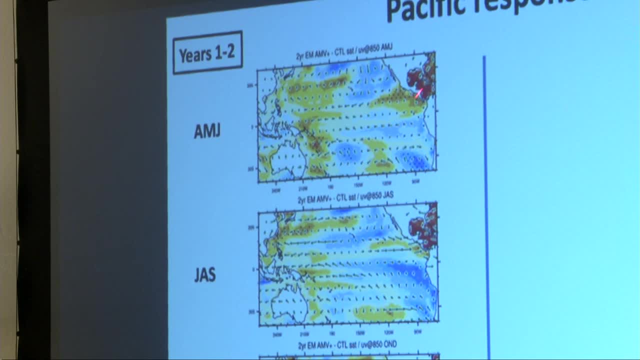 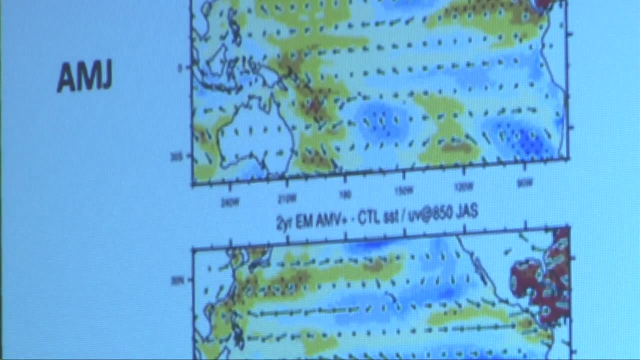 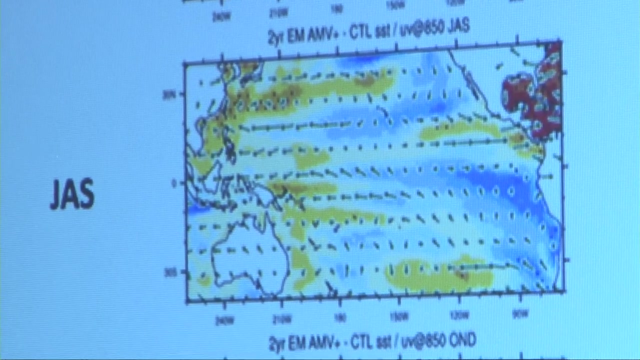 So basically the time is going like that. So we can see that in AMD we can just see a little warming over the eastern Pacific there And with time we can see the emergence of cooling over the Pacific, Over the cold zone there that is propagating westward to the central western Pacific with 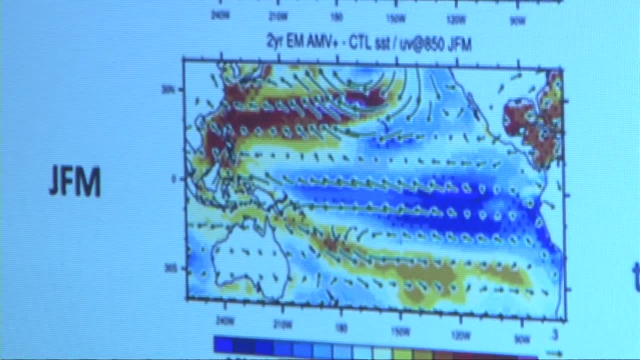 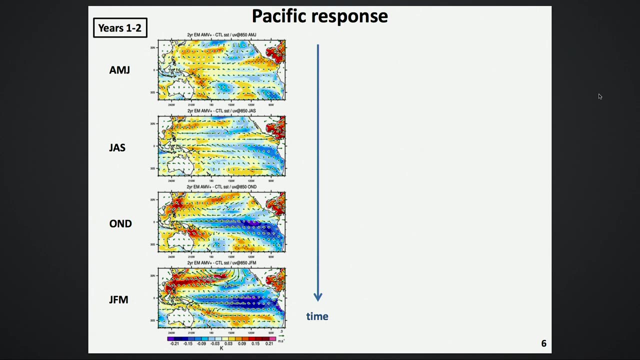 time through a complete linear type signal in GFM. So to understand how this- yeah, linked to this cooling there is a wind antibody, So I guess you can't really see the arrows there, but there is an increase of the trade there. 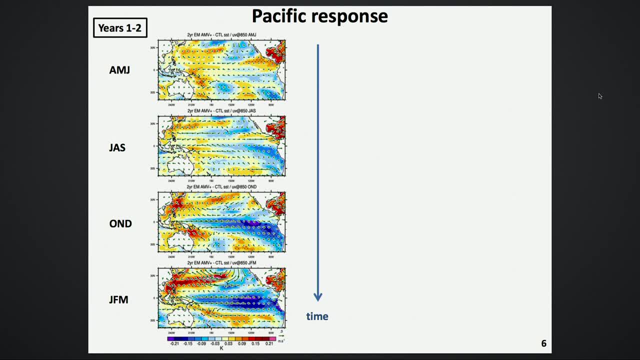 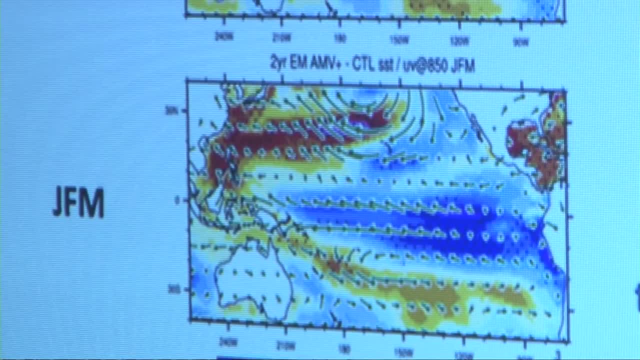 So we can see that in GAS and that's a stress in October, November, December and then strong increase of the on the trade in GFM. So to understand how this happened, I need this map that are basically the same as this. 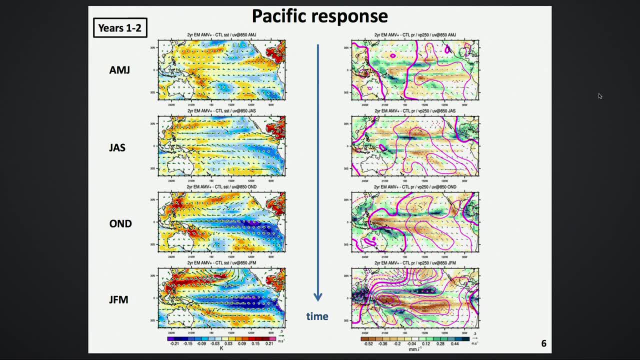 one, but for precipitation in color, and the control represents a velocity potential at 250 hectopascal. So we can see that in GAS we've got a subsidence anomaly over the Pacific here. That's, yeah, Okay, And indeed it's caused by an increase of the precipitate, of the convection of those. 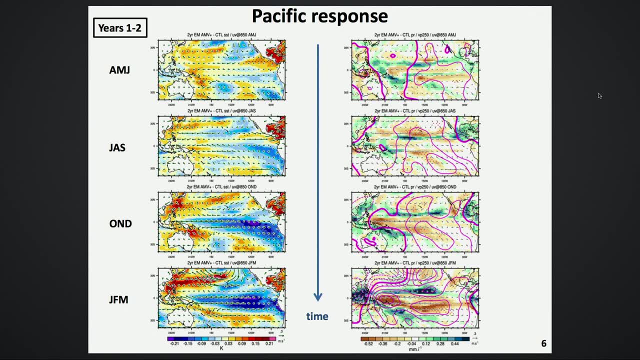 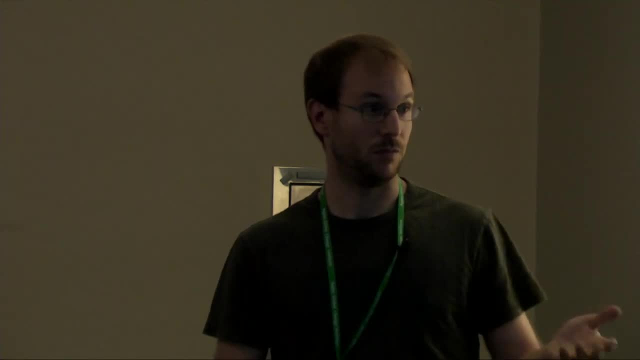 tropical Pacific over the Atlantic- yeah, That subside here- And this is going to increase the trade over the central and the western Pacific and, finally, is going to create this linear type response that we can see both in SST and precipitation there. 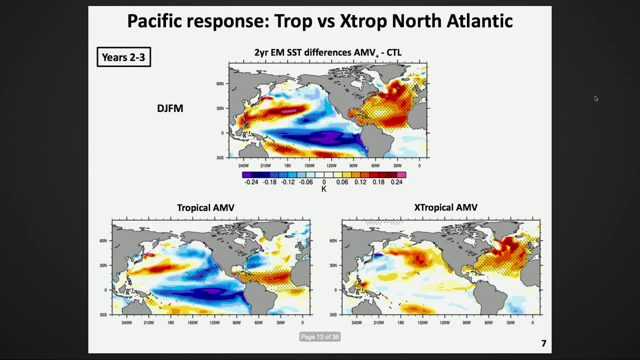 Okay, So yeah, Thank you, Thank you. So, as I said, we try to understand that this influence is due to the extra-tropical part of the tropical part of the MV. So we did two extra experiments: One where we restore only the SST, the MV SST over the tropical part, and another where 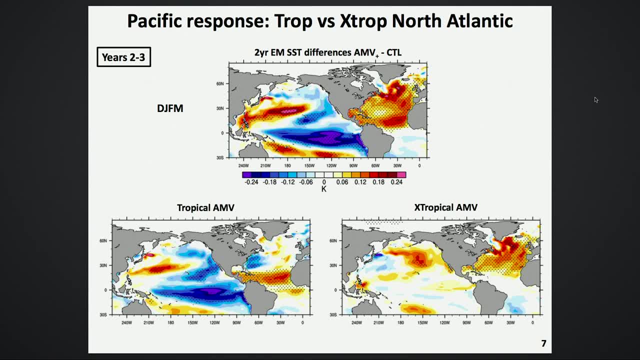 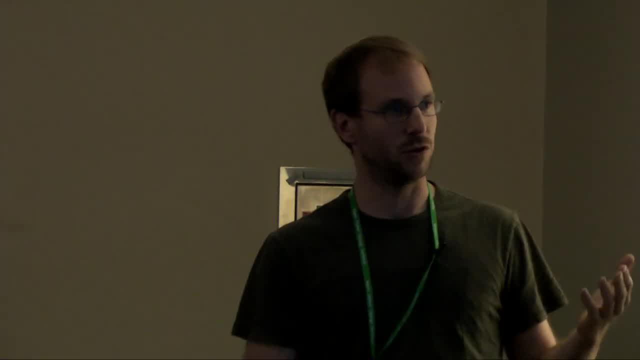 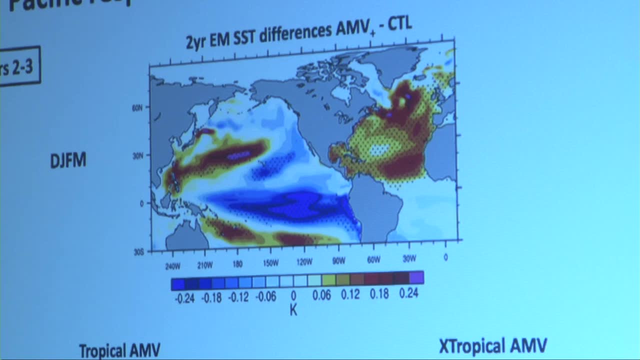 we only restore over the extra-tropical part. So here is the map for it's SST. different in DGFM between the MV plus experiment and the control simulation. still, And it's the same for these two different maps. but anyway, And I focused on the two free here. 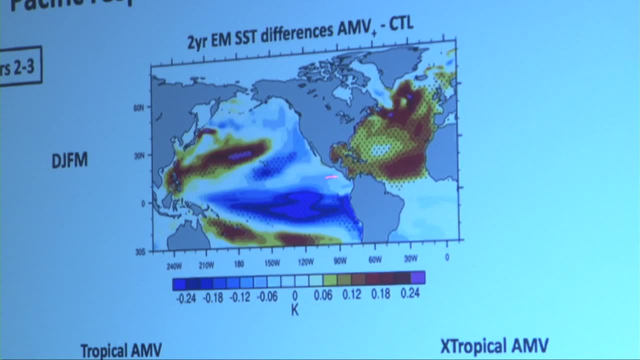 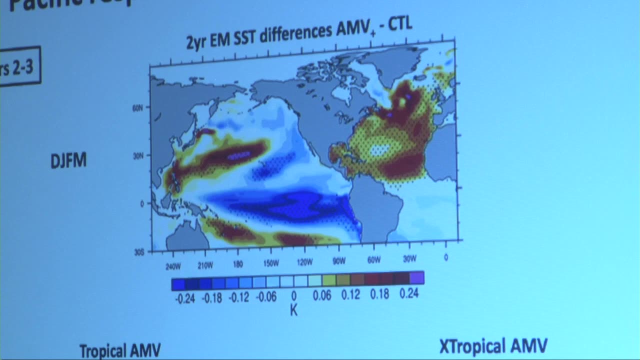 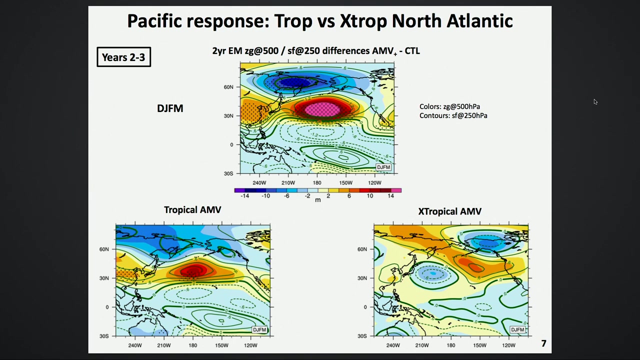 So, basically, what you can see is that the signal here is mainly explained by the tropical part of the MV. Yeah, If we look at this, the atmospheric circulation, we've encoded the zero potential at 500 watt. extra-tropical, Yeah, Okay. 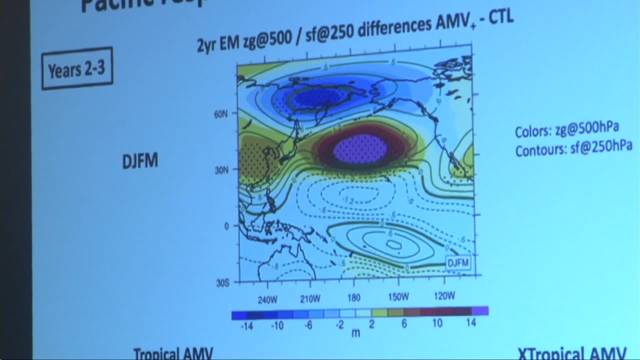 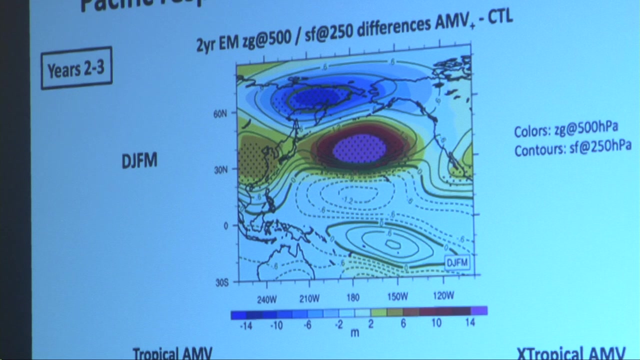 And in control the stream function at 250 hectopascal. So we can see that there is this reduction of the ocean low over the Pacific there And it seems to be coherent with extra-tropical tropical tropical, extra-tropical Roseby wave. 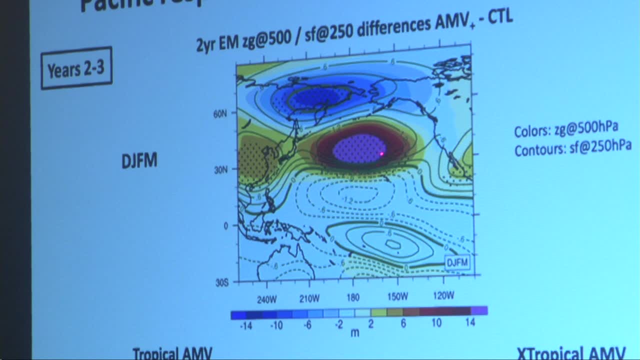 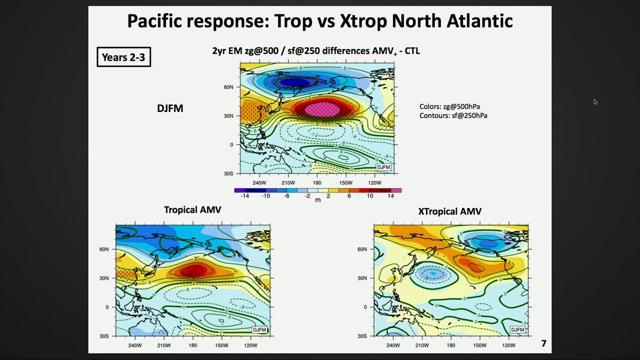 anomaly, As we can see. we can follow kind of a wave trend between tropics and extra-tropics there And we can see that this, this anomaly is As well. it is present as well in the tropical MV experiment, but not in the extra-tropical. 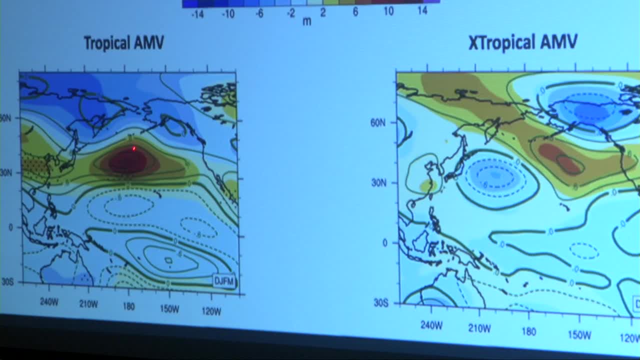 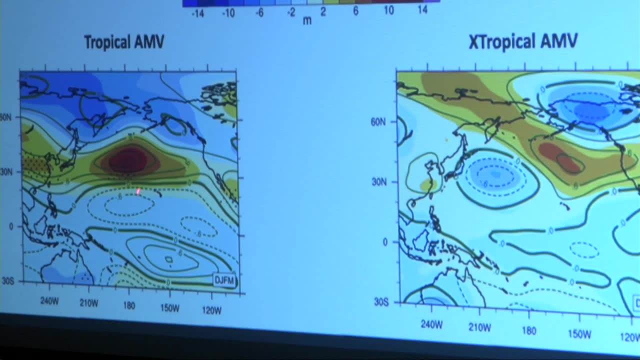 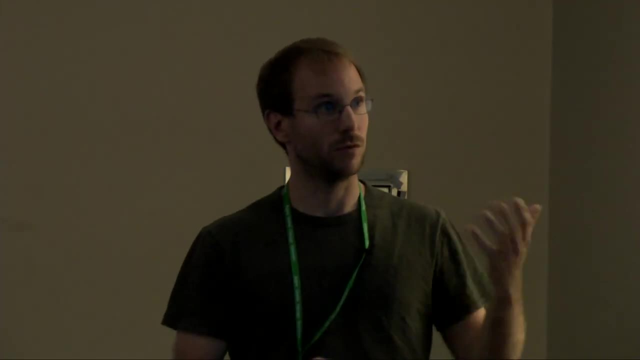 MV. So yeah, the amplitude is bit lower in the tropical MV comparing to the full MV experiment. This suggests that this mechanism is led by the tropical tropical MV. but we need that all the North Atlantic warming to to get this strong response there. 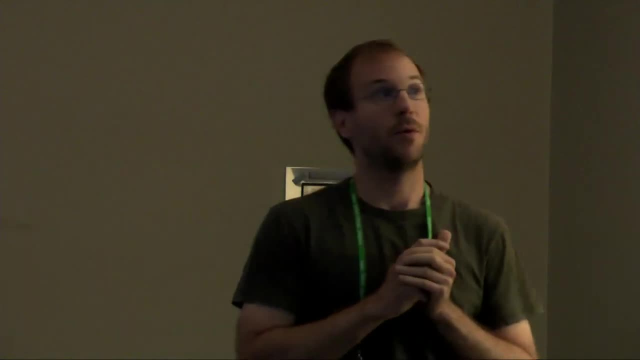 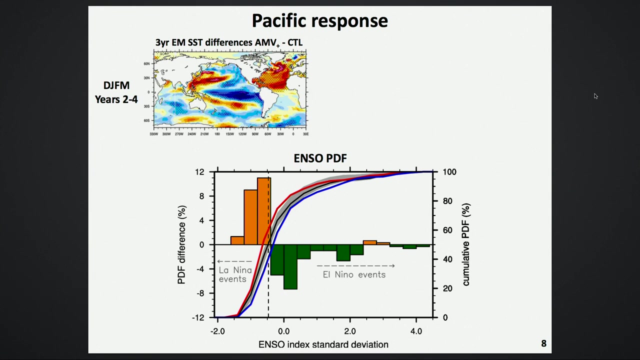 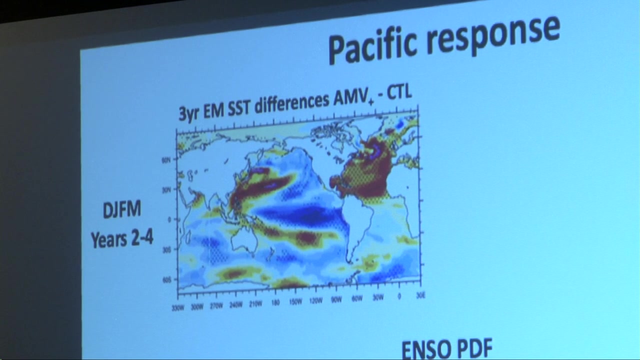 Okay, Yeah, So, okay. So now I show how this, this anomaly happens there. but I'm going to to to show you that this, this tropical response, is not stationary. So to do that, to do to show, to show that what I am going to focus on, the density, the 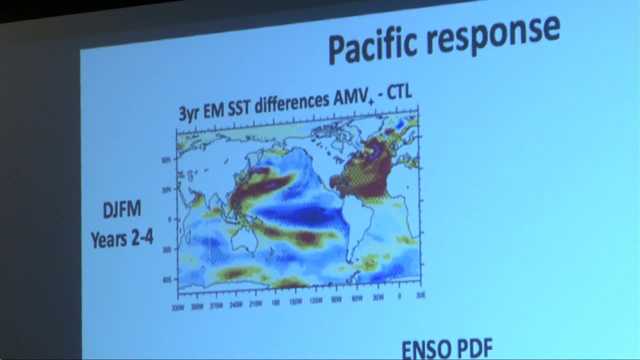 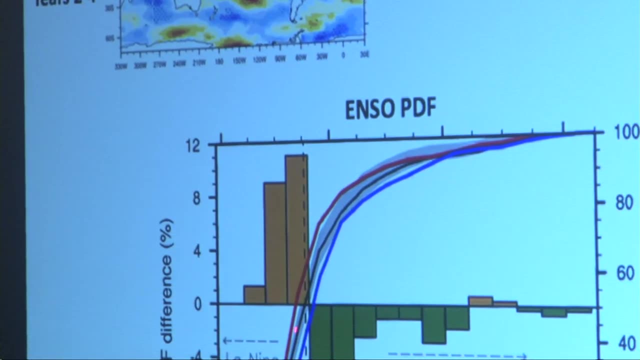 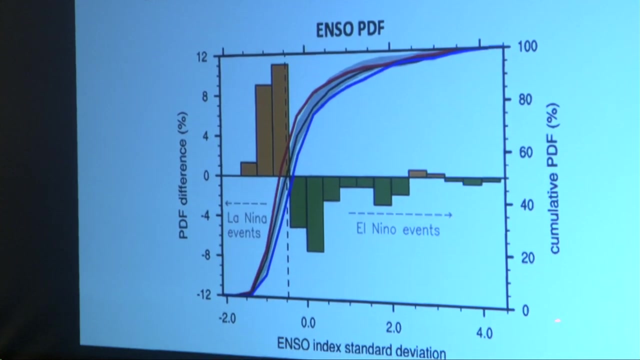 probability, the density of, of probability of the ENSO in the experiment. So this is represented by this graphic here. So the black line here represents the cumulative PDF of the control simulation. So, going to 0%, 0% to 100%, and we are going here from Laninia event to El Niño, to El, 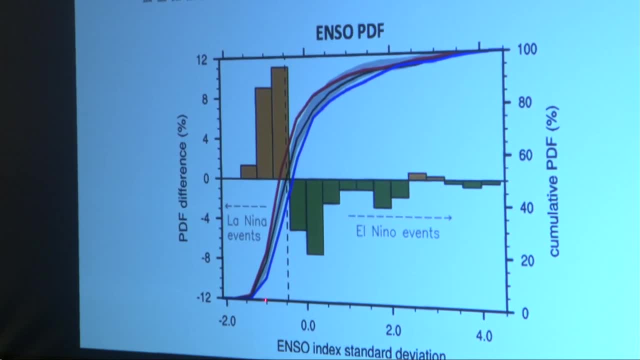 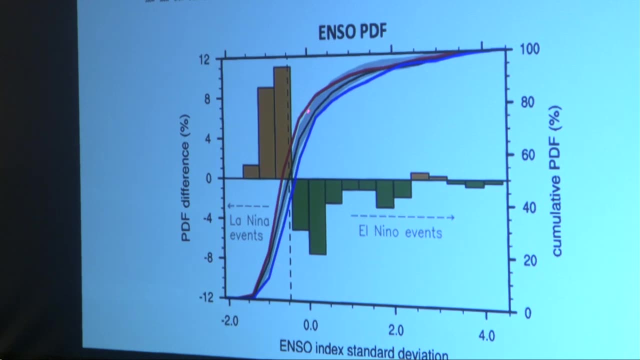 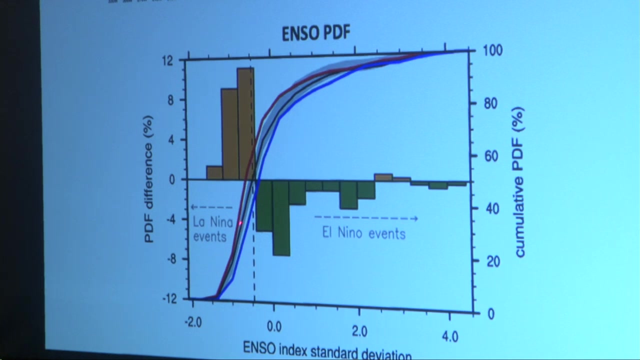 Niño event there And the red line represents the cumulative PDF, but for the MV plus experiment. So we can see that there is more Niño event in the MV plus experiment comparing to the control simulation, And the blue line represents the same thing, but for the MV minus experiments. 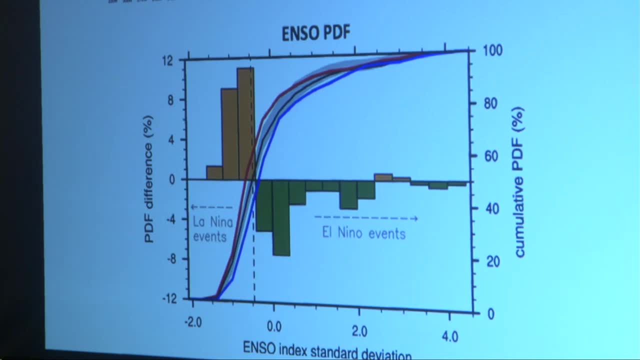 So basically, it's the opposite: We've got more Niño events in the MV minus, MV minus experiment. I forgot to tell you, to tell you that this gray shading here represents the confidence interval over this, this cumulative PDF, And the histogram here represents the difference, bin by bin, between the IMV plus experiments. 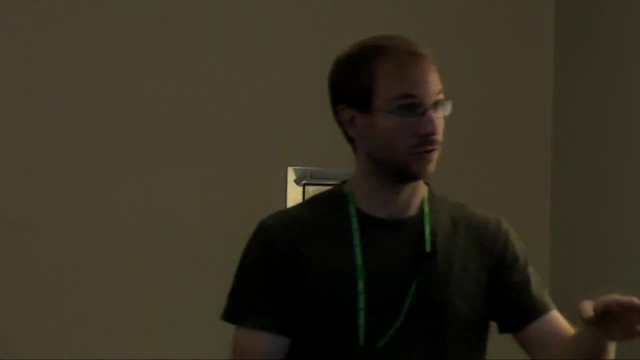 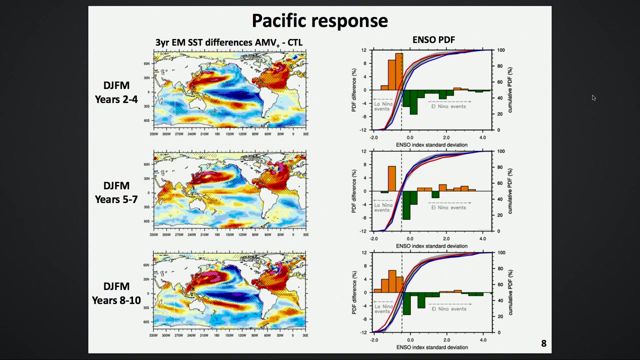 and the MV minus experiments. So I'm going to use this graph in the next slide to compare different period of my simulation. So here is for year two to four, here for year five to seven and here for year eight to 10.. 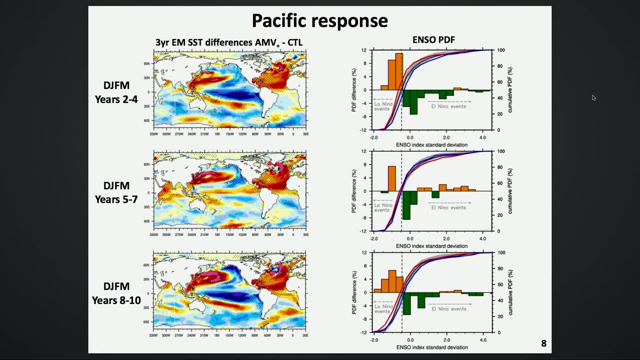 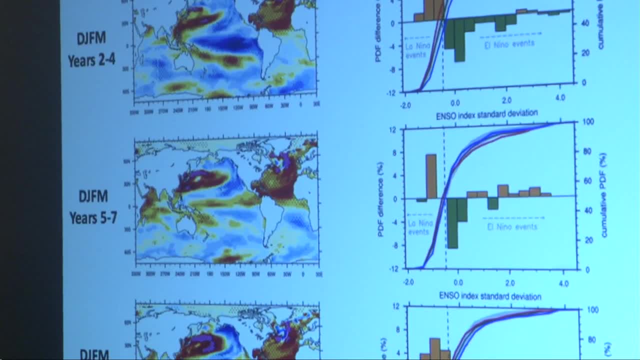 So you can see that there was a cooling during these years, but then it's followed by slightly warming of the tropical part, the Pacific, And then we are going back to Niño condition And indeed, if we look at this PDF graph, you can see that there is a cooling, but then 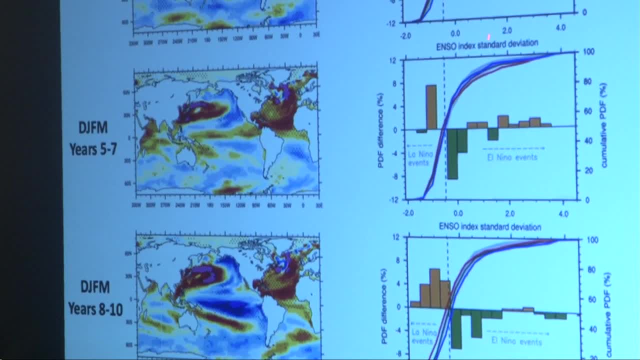 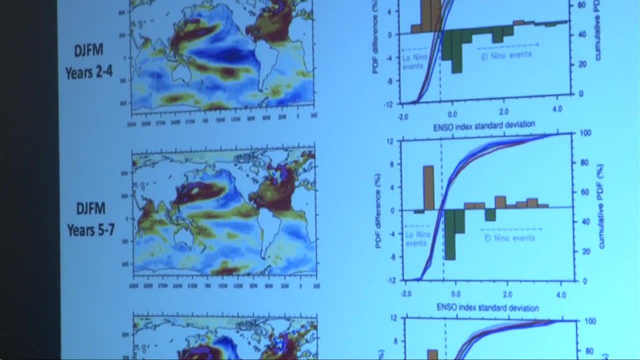 it's followed by slightly warming of the tropical part, the Pacific, And then we are going back to Niño condition. So here we have a graphic. We can see that the red line and the blue line switched and they are just the opposite. 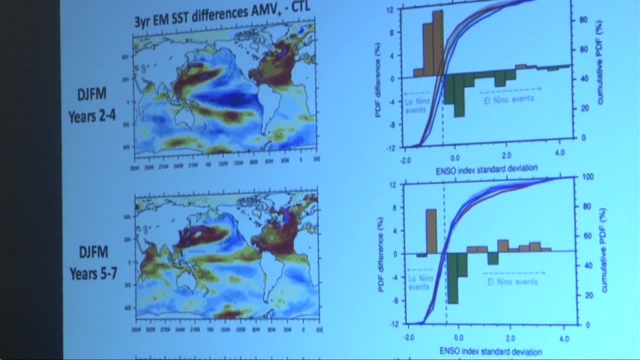 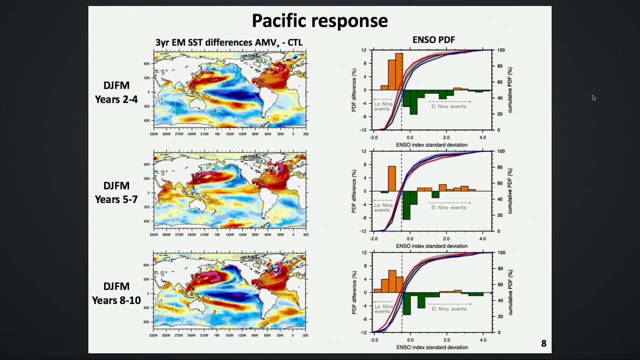 of what was during this year, so during the year five to seven. So that suggests that during this year there is finally more Niño event than Niña event in the MV plus experiment, comparing to the control simulation. And finally we are going back to the same thing at year eight to 10.. 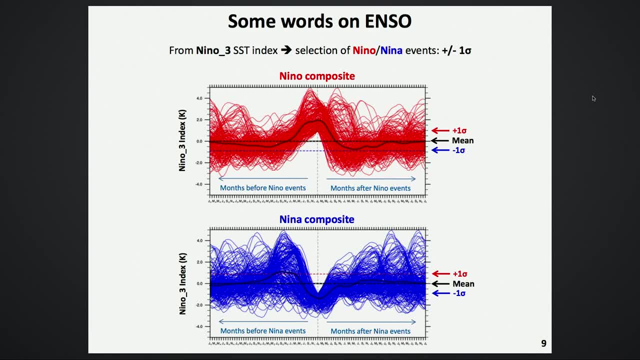 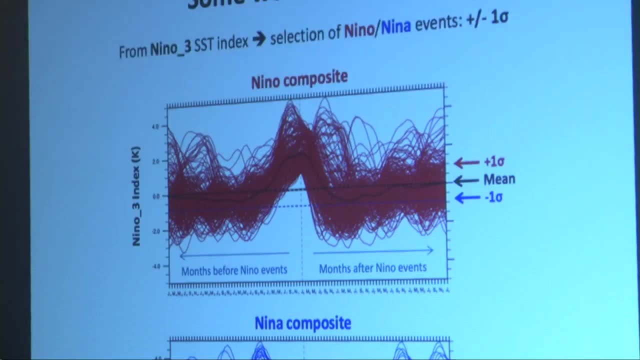 So I try to understand why this happened. Is there also predictability and ENSO? But so to understand why this happened, I have to say some word of ENSO in this model and of ENSO in general. So what I did here is I computed composites. 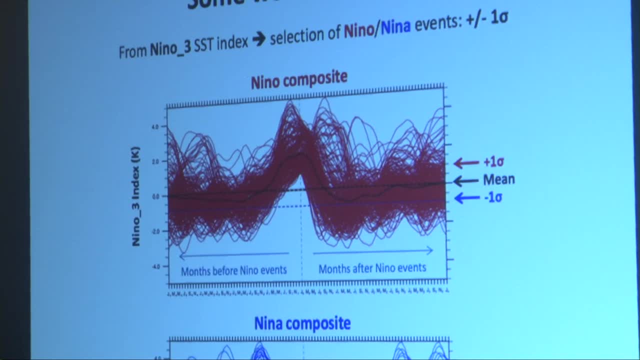 of the NINEO-free SST index in my control simulation. So I select the NINEO and NINA events based on a threshold of plus or minus one standard deviation of the NINEO-free SST index. So here's the dashed line represents: 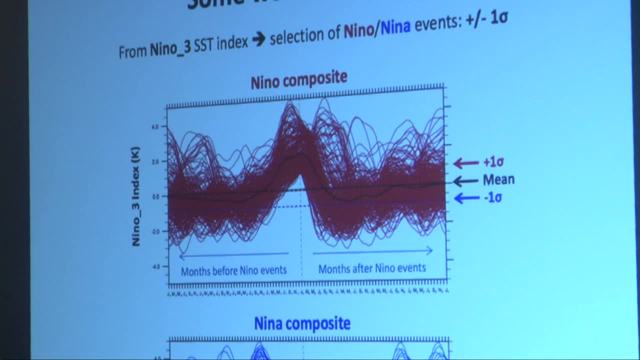 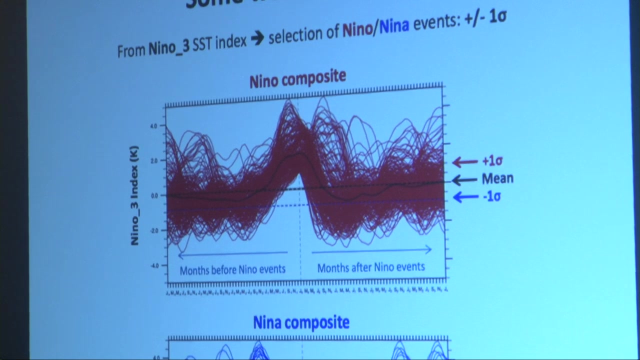 the maximum of the NINEO events that I chose for January And every line represents all the different events that I obtained. So we can see that some event peaks before January, some peaks twice in January and then the next year. So there was a lot of different behavior. 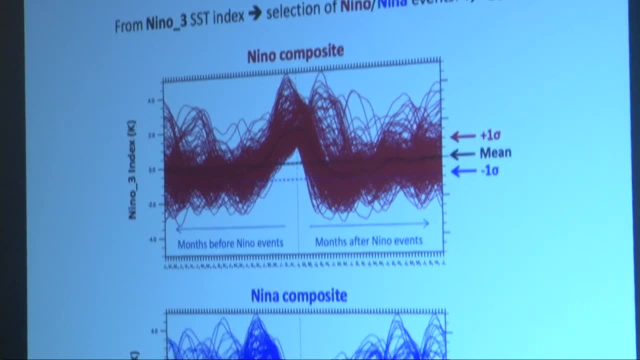 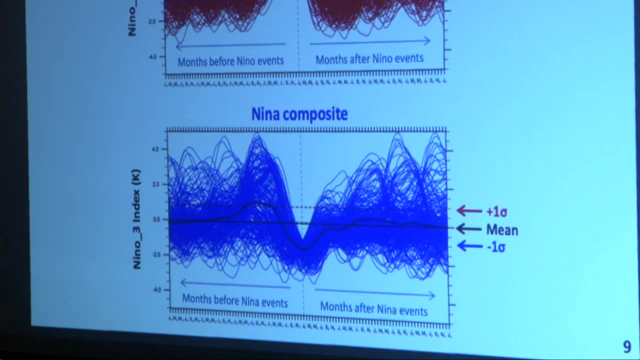 in all these events. but here I just want to focus on the canonical ENSO behavior. So I did that by computing the ensemble, the mean of this composite that is showing in bold lines there. So if I only keep that so I've got this line. 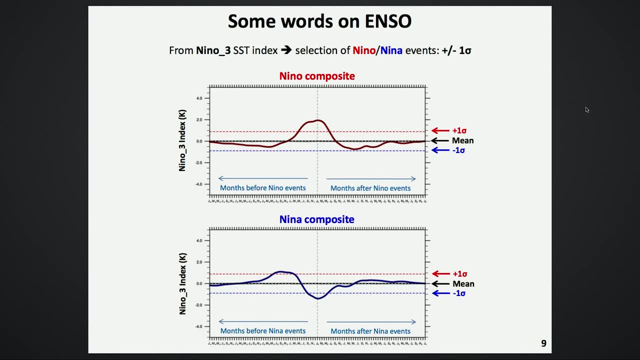 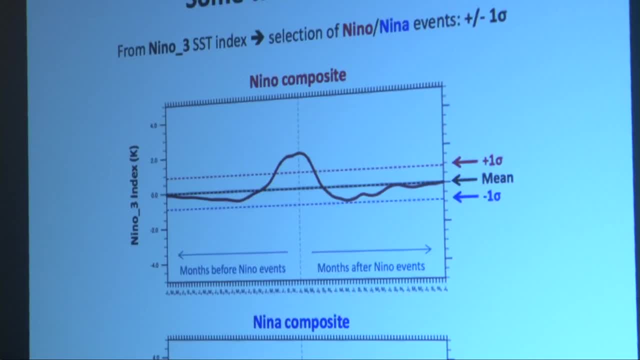 so we can see that after NINEO events we then go to cooling. that seems to stay for at least two years there. Yeah, here's the time in months, Right? and for NINEO composite we can see that after NINEO composite there is finally a warming. 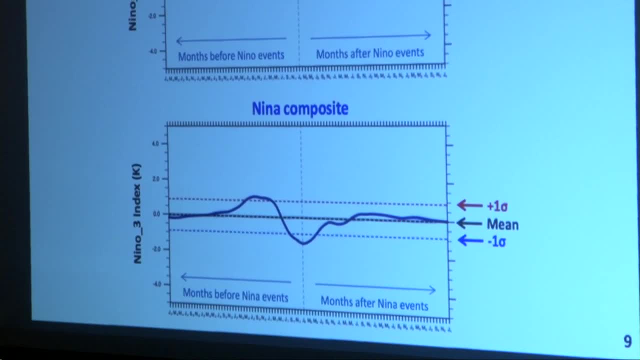 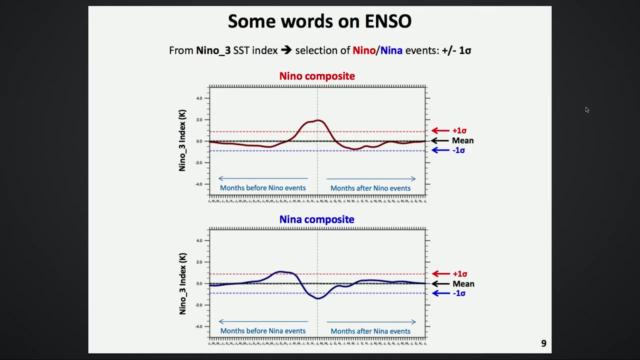 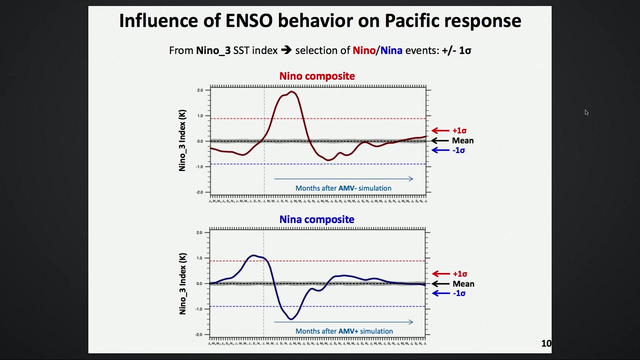 a slight warming, but still a warming of the tropical, of the NINEO-free index, NINEO-free zone here during two or three years. So how this can be related to my experiment. So now this represents a NINEO-free index. 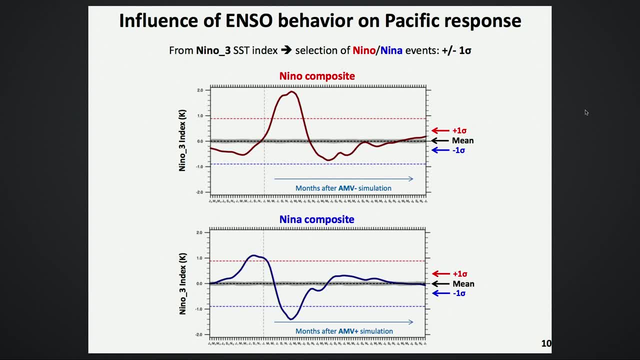 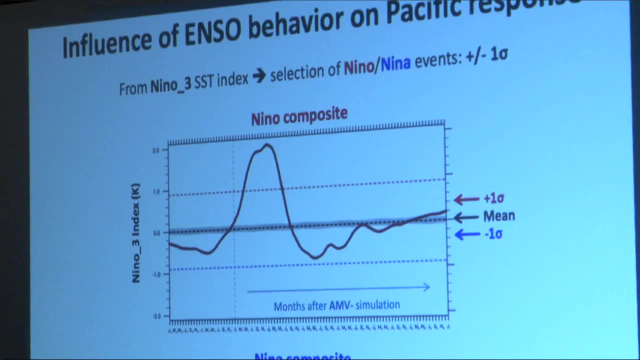 in on here, the dashed line represents the starting date of my simulation. So as we saw that there is more NINEO events in my MV-minus experiment during the first three years, But what does it mean concretely? So here I represent one number that got the same behavior. 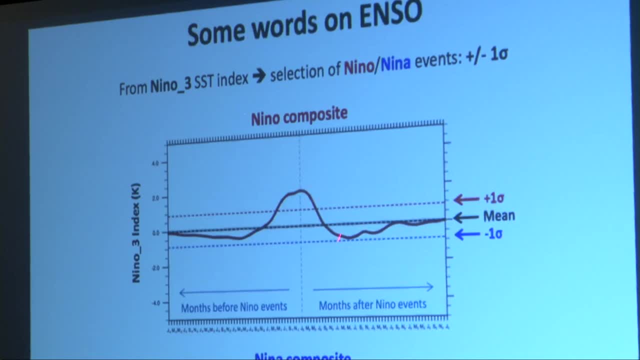 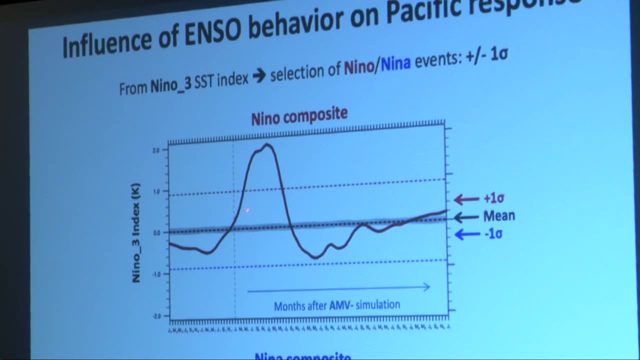 that sorry than this canonical ENSO here. So it just, I just represent the same thing here, but just zoom in So you can see that if one number show NINEO, a NINEO event is not going to be warm for three years. 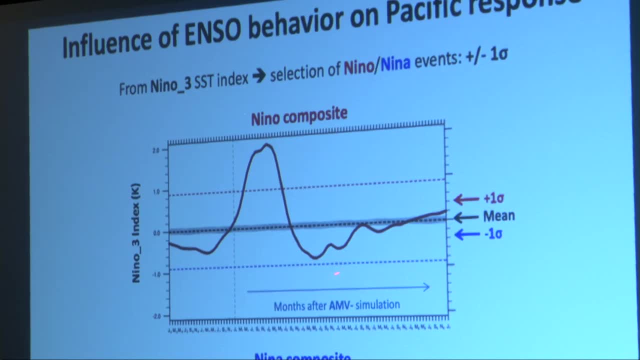 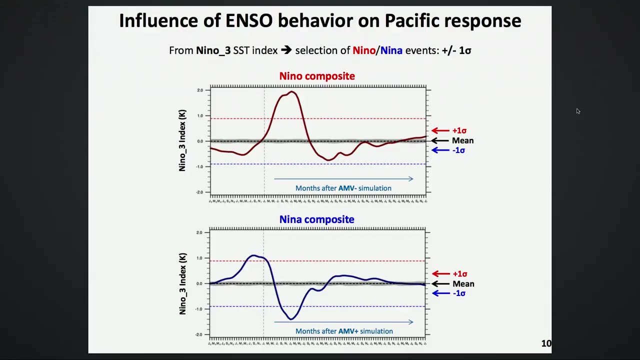 what's happened is going to cool down after the first years and then it's going to show cooling. So if there is warming during the first three years of the experiment, it's not because only one of all members that show warm condition during the three years. 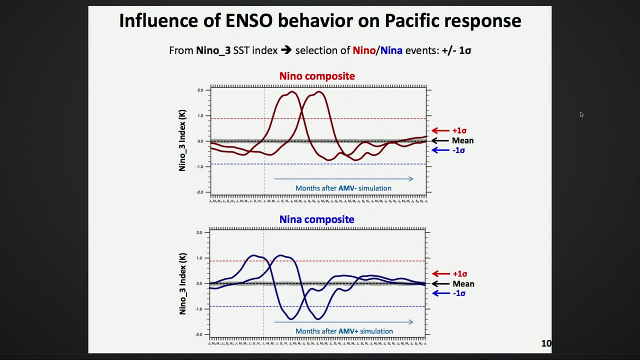 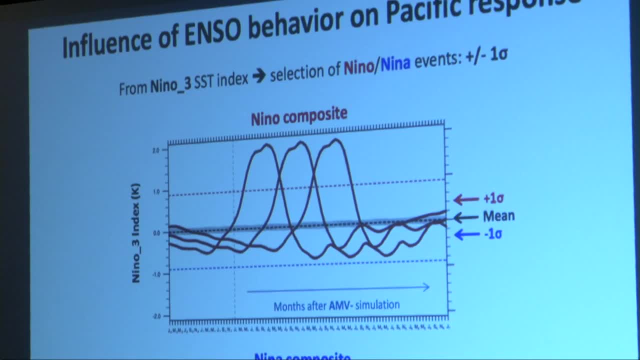 it's because there is warming for one member over the first years and then another member is going to show a NINEO event the second years and et cetera, And another member is going to show that. So when I average over the three years, 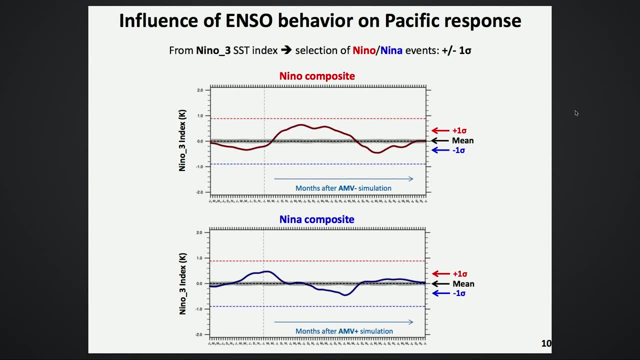 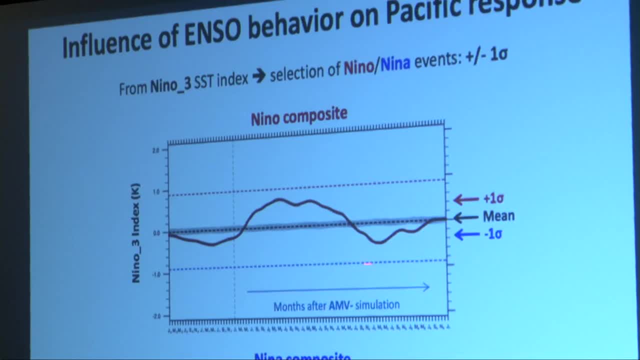 and I average over all the members. I obtain this kind of residual and we can see that there is a warming here during the first three years of the simulation and then it's followed by cooling And for the NINEO composite. so that means the MV-plus experiment. 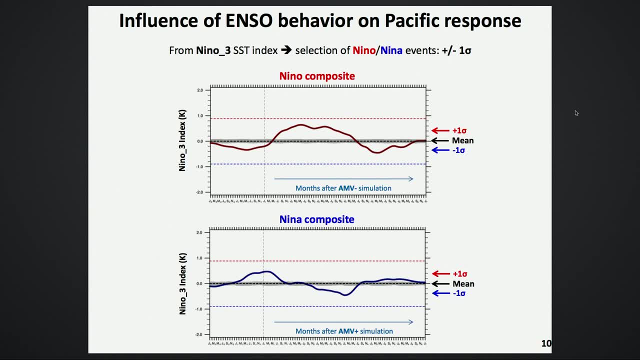 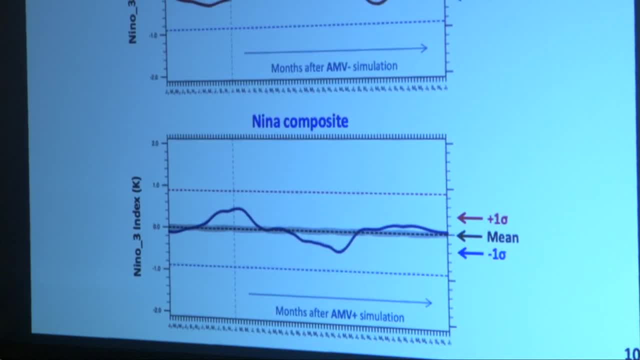 it's similar. there is cooling over the first three years and then it's followed by weak warming there. So this- this is This- is done by just hand. So is it really what's happening in my simulation? We have to test that. 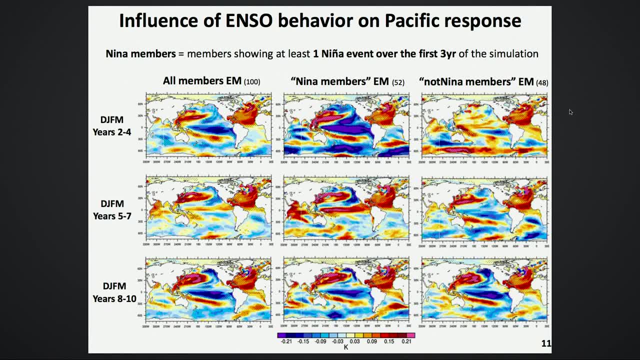 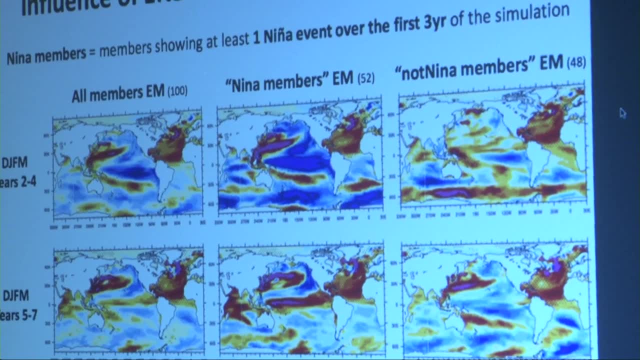 So what I represent here, it's still the SST ensemble, mean difference between the MV-plus and control simulation in DGFM for the year two to four. So as you already seen before, Okay, on year five to seven, eight to 10.. 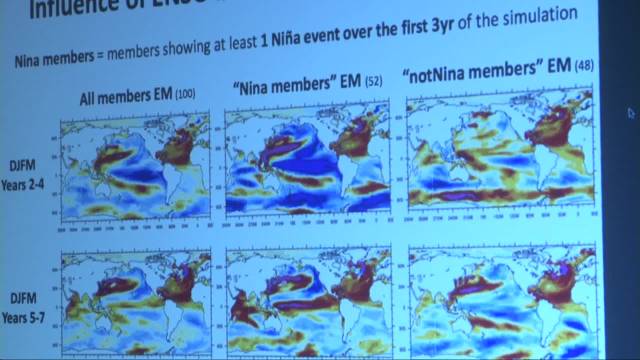 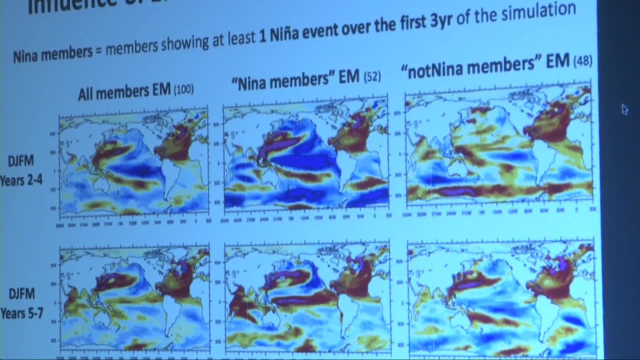 And here it's the same thing, but for a sub-sampling of the ensemble members. So I choose only the NINEO members. So what I call NINEO members, it's the members that show at least one NINEO events. 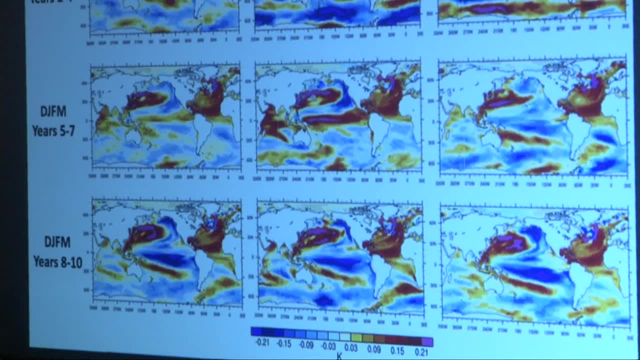 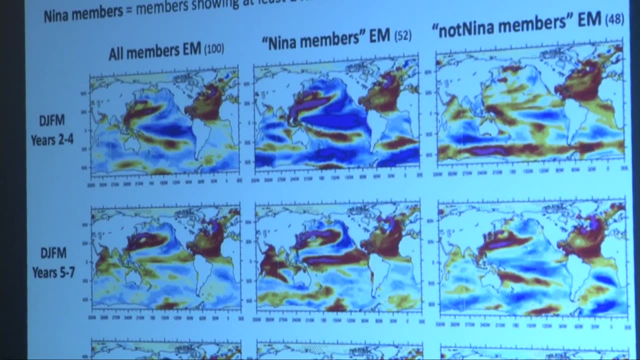 over the first three years of the simulation. So by construction I've got a strong cooling over the first three years here. But what is interesting is to show, to look at their evolution, So you can see that there is after this cooling, there is finally warming. 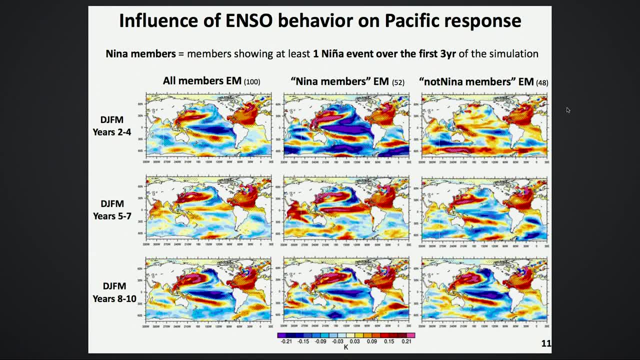 And then we're going back to NINEO condition. And if I do the same with the members that doesn't show NINEO events during the first three years, then we're going back to NINEO condition And if I do the same with the members, that doesn't show NINEO events during the first three years. 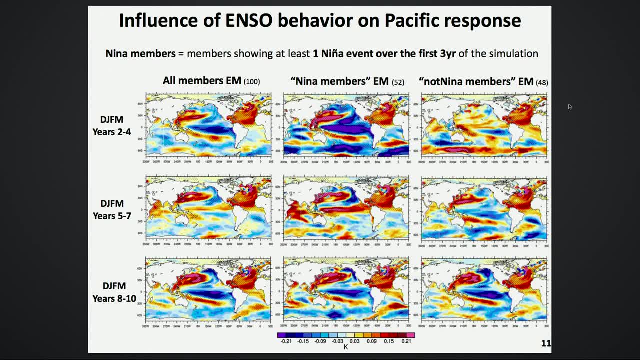 finally, we can see that there's no cooling at first And then there was weak cooling in the first five to seven and then NINEO condition. So this suggests that the switch between NINEO to NINEO. So this suggests that the switch between NINEO to NINEO. 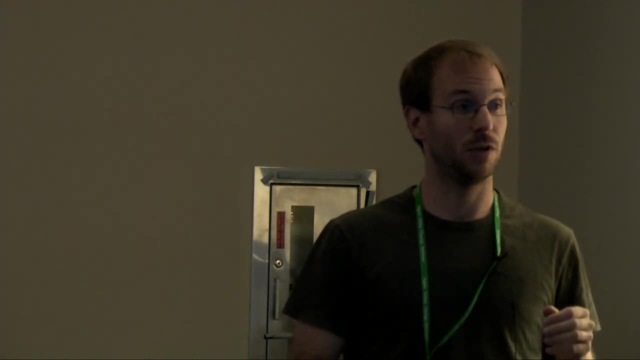 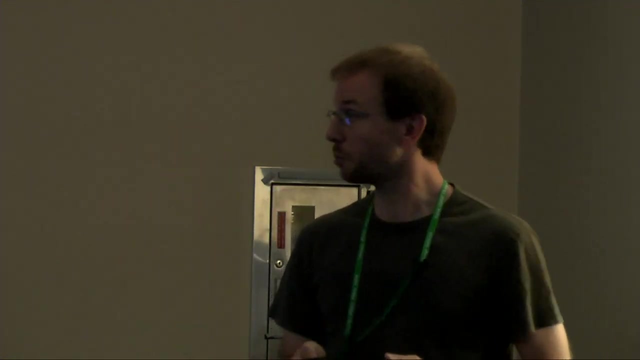 So this suggests that the switch between NINEO to NINEO and then to NINEO condition in this experiment is indeed due to the ENSO behavior. Oh, thank you. Okay, Okay, Okay, Okay, Okay Yeah. 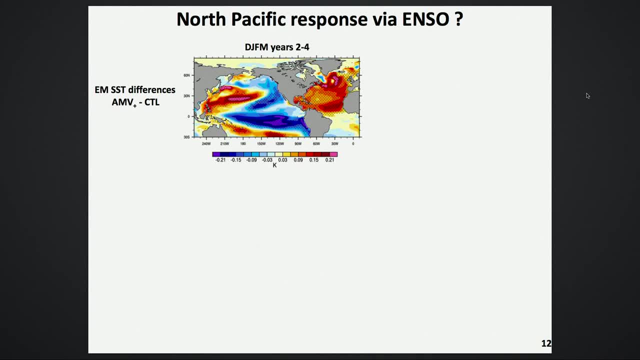 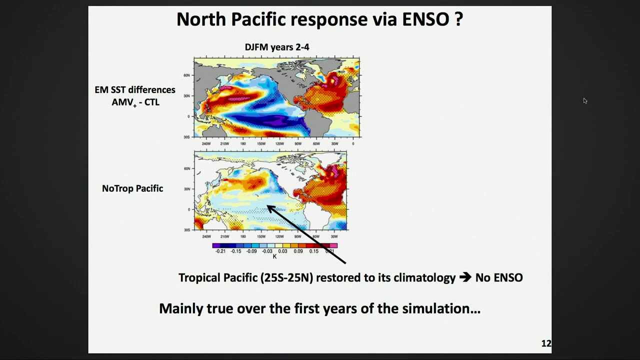 That's it. So now I want to ask: does the North Pacific response here is effectively due to the ENSO response? So to do so, I did an additional experiment where I restore the North tropical Pacific to its climatology. So I just cancel ENSO here. 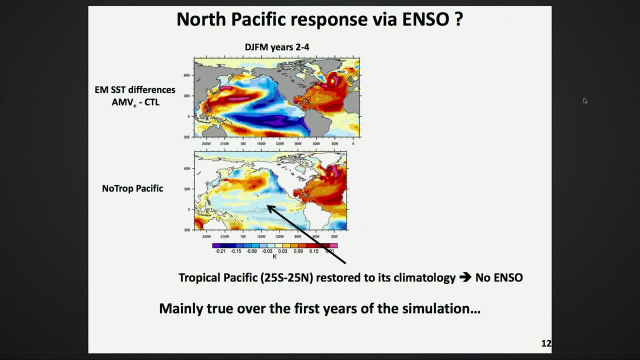 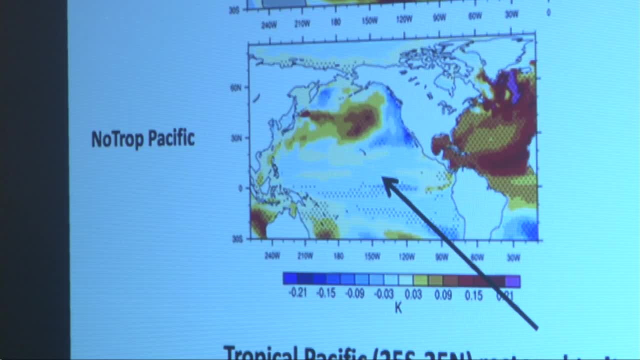 And what you can see is that the North Pacific response is mainly due to the ENSO response And so anomaly that occurred in the tropical part here. So this is true for the year two to four, But if we look at longer time scale, 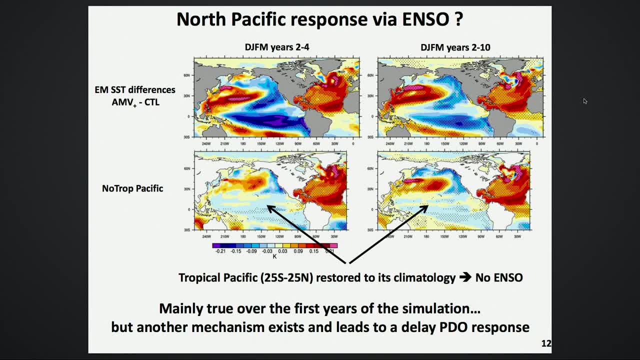 so if I average over the 10 years of my simulation, so there is this PDO kind of like response here. And finally we can see that even in this experiment we still have this PDO response. If I look at the extra tropical North Atlantic. 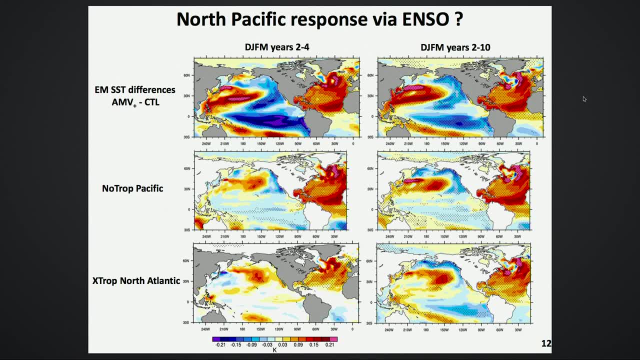 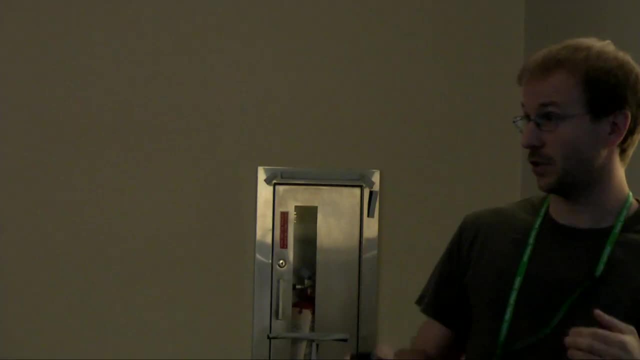 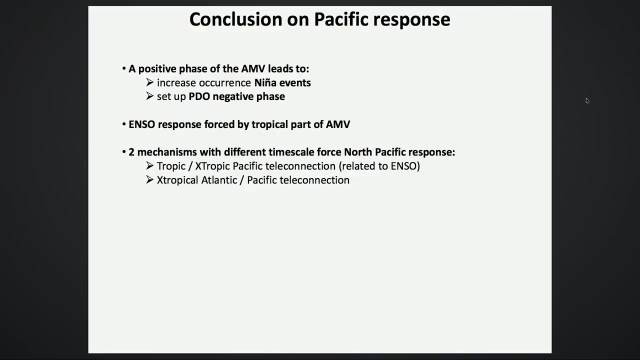 So this suggests that there is another teleconnection between the Atlantic and the Pacific that is caused by the extra tropical part of the Pacific. So, yeah, so here's the conclusion of my talk. So we saw that a positive phase of the MV leads to an increased occurrence of the NEA event. 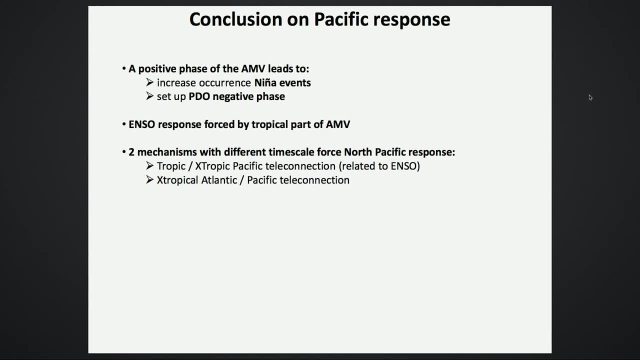 in the first years, And then as well, to a setup of a PDO, of a negative phase of the PDO, We saw that the ENSO response is forced by a tropical part of the MV, whereas the PDO response is forced both by a tropic 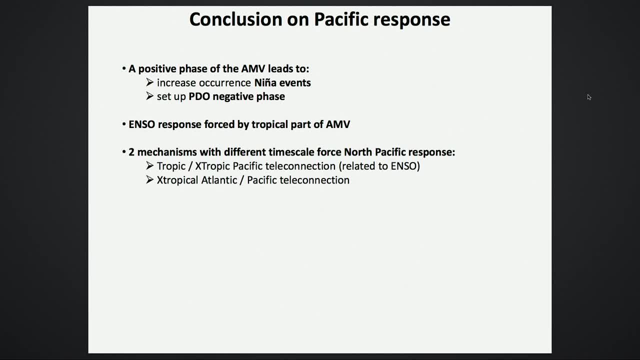 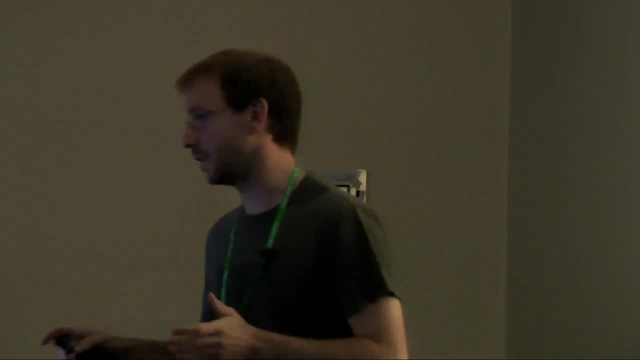 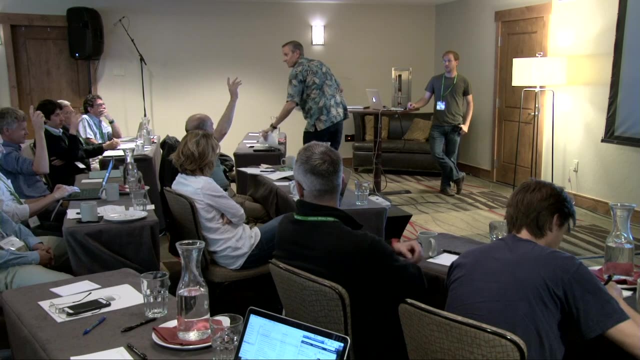 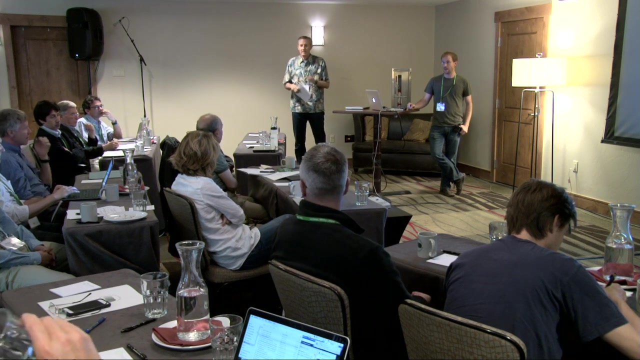 extra tropical Pacific teleconnection, so related to ENSO, but as well to a extra tropical Atlantic Pacific teleconnection. So that's it, Thank you. Thanks, Any questions? I think it's a very nice demonstration of how ENSO really interferes with longer timescales. 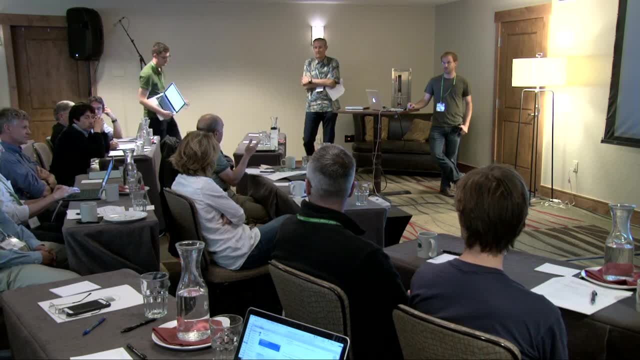 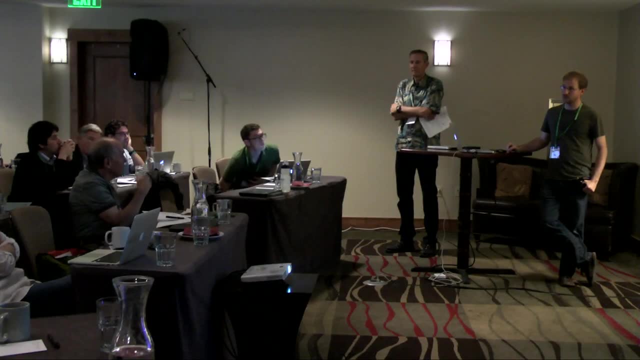 And because you are setting up this experiment as a startup experiment, then you're actually getting a mix between the ENSO tendency to have some sort of a cycle. I think it was a very nice information, But what I wanted to say is that Axel Timmerman has already 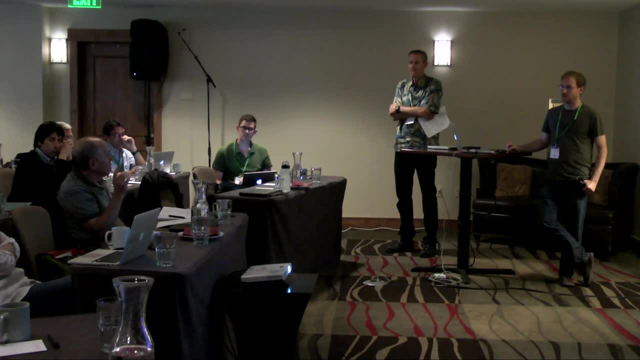 pointed out earlier that what happens because of the AMO in V is that you tend to get that intensification of the trace and lift the thermokine and then tend to get the preference for La Nina conditions and that sets up the internet. And the last thing I want to do is: so, if that works like that, 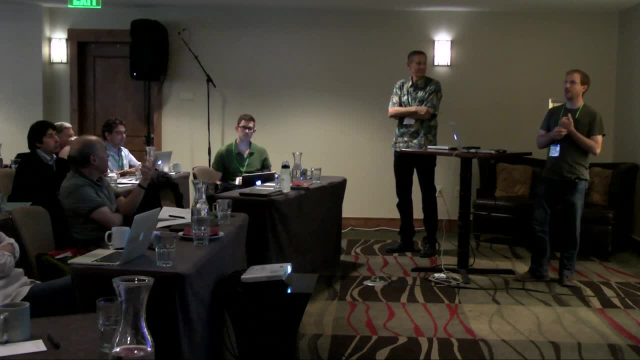 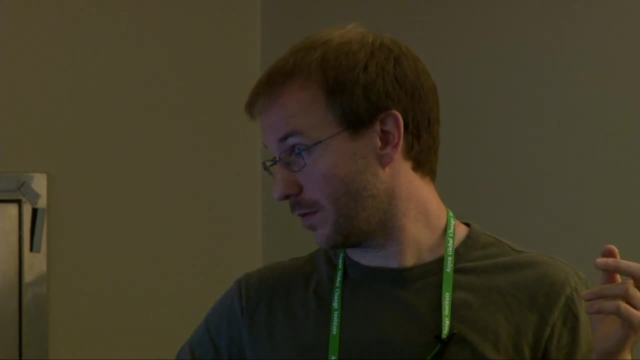 why don't we get predictability in the Pacific from? we do have predictability in the AMO, so why don't we get predictability in the Pacific? One possibility is because. so this is a pattern that we're imposing in the simulation. 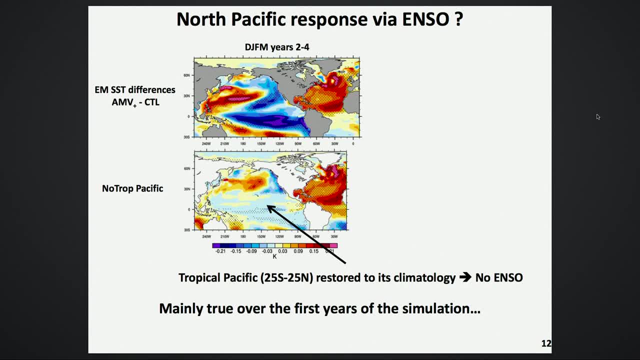 So we've got this strong tropical warming And in the couple model the AMO doesn't show this strong warming. here In the model. usually you don't get that. Yeah, it's not so strong, So this could explain why there is not. 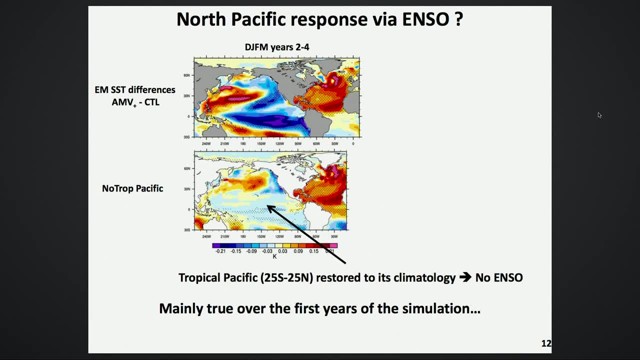 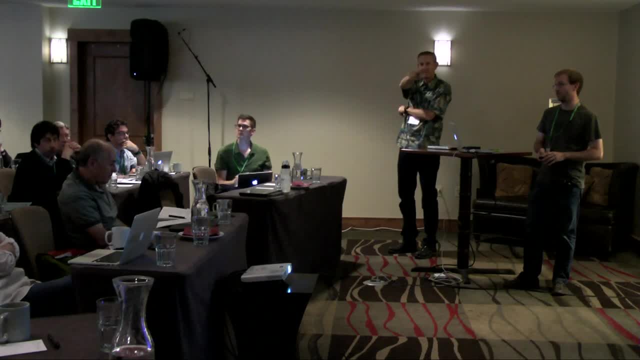 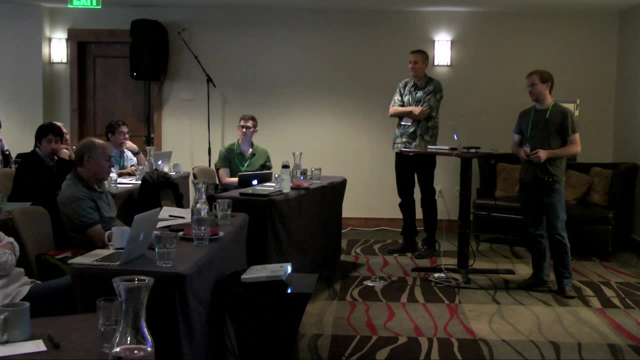 this tropical, So maybe we lost this predictability on the North Pacific alone. It would be better, though. So it's a fascinating question. Yeah, So there's a lot of, So I have two small questions, So one: did we get the very first winter response? 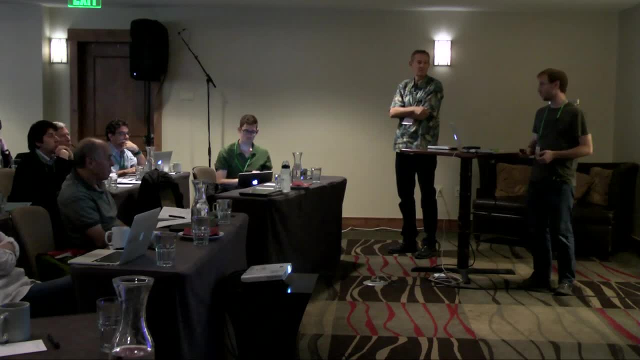 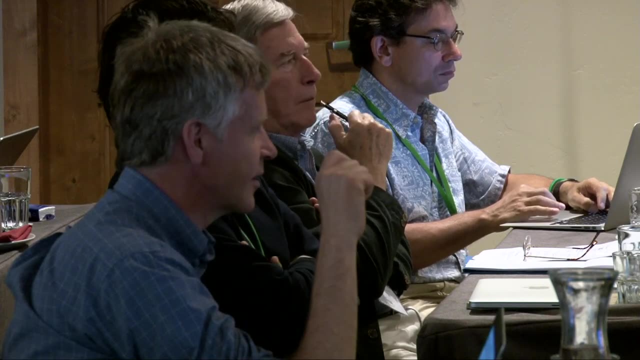 in terms of seeing the pressure to see anything in the AMO The first winter, The very first winter, So I don't have time to show that today. But yeah, we wish, Can I show this plot? Yeah, Yeah, cool. 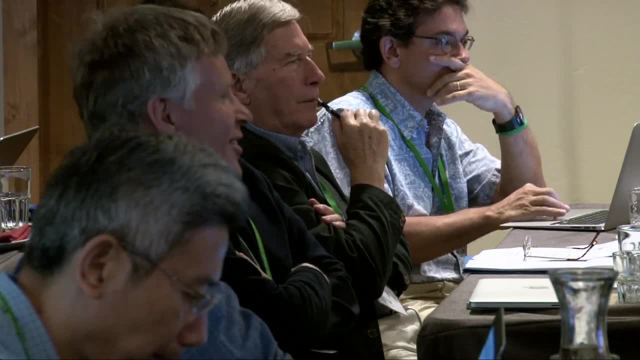 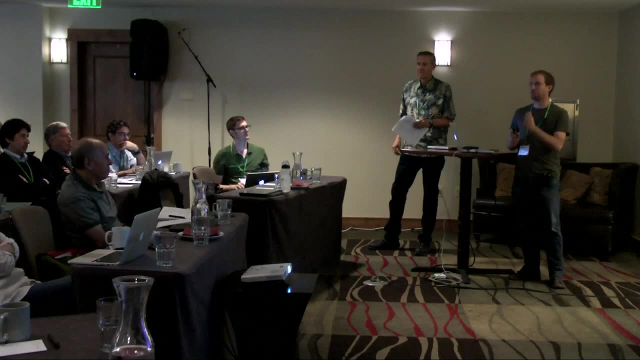 That was presented, though, OK, Sorry. So the other one was this fascinating. But yeah, there is definitely something, the loss of the Atlantic, but it may be high by something that's cold. So what is the mechanism for that? 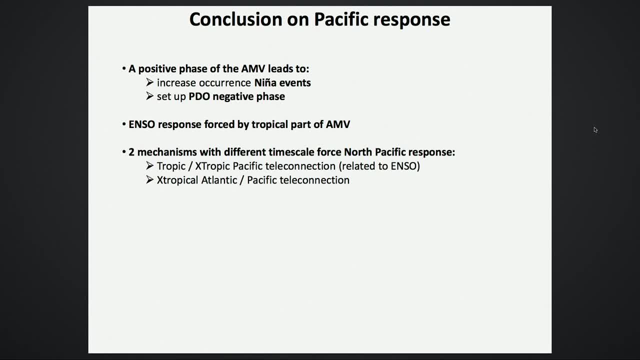 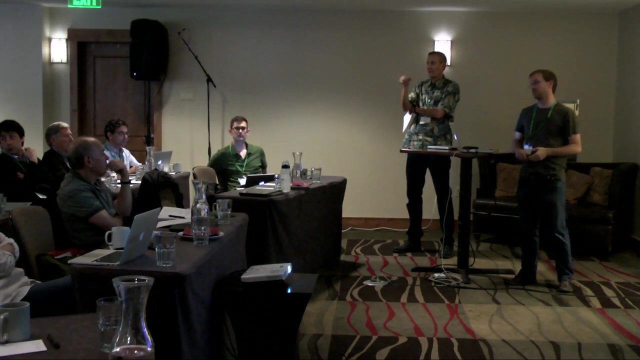 We still didn't work so much on it, But I think Zong- and that was in 2007,- explains this mechanism by the storm track activity that may link the exotropical part of the MV to the exotropical Pacific. I'd like to ask about the metrics that you used. 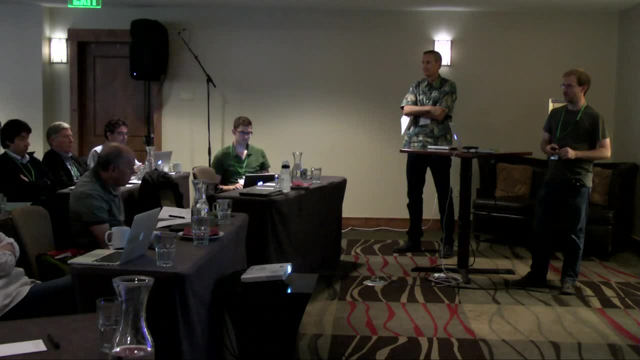 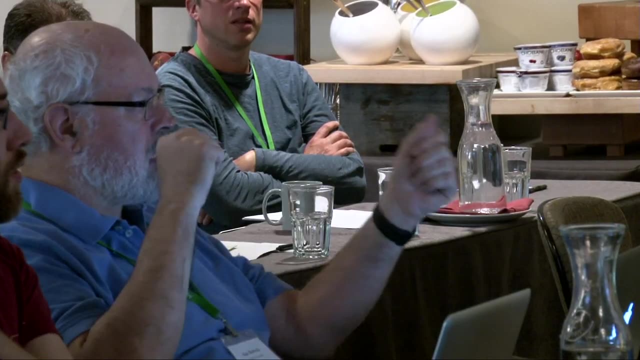 because it might be different from other people and it might make it hard to compare. You used DJFM in some of your figures. You used JFM in other figures. How did you decide how to define the season? And also you used NEO3 rather than NEO3.4,. 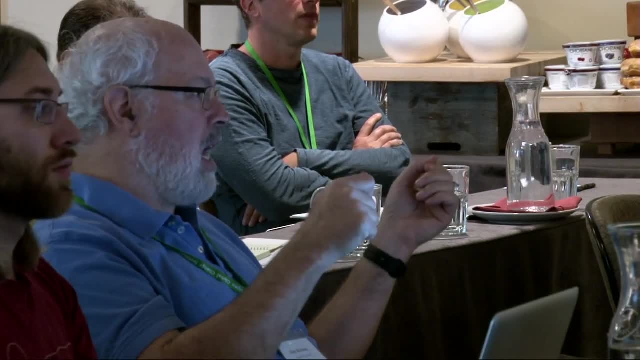 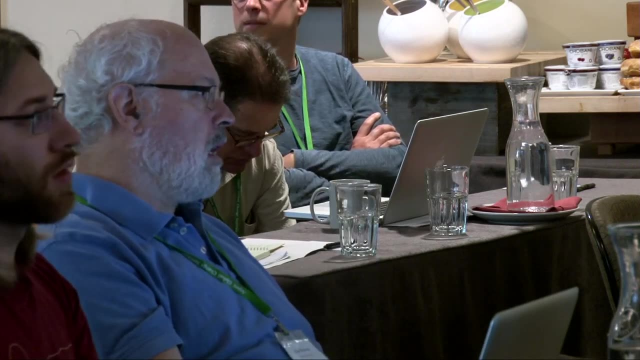 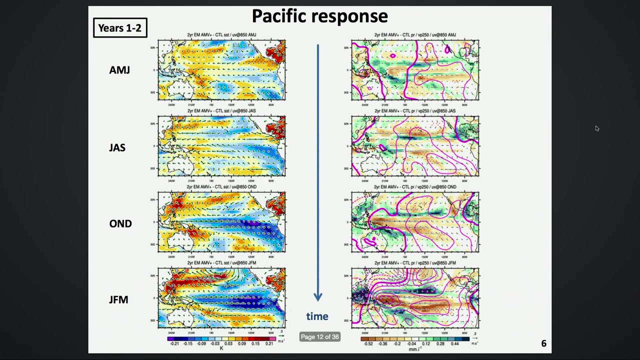 which is more conventional. How did you decide to use that to define the NEO? Because if you're comparing to other people, they use different metrics. It might be confusing. So for the season I just drew once, only three months- It was just for this thing here to understand. But why didn't you use DJF, which is the traditional metric definition? The only reason is because I just picked the year in three months and that was the only reason for that. For the DJFM, Well, the traditional season definition for winter begins on December 1st, not January 1st. 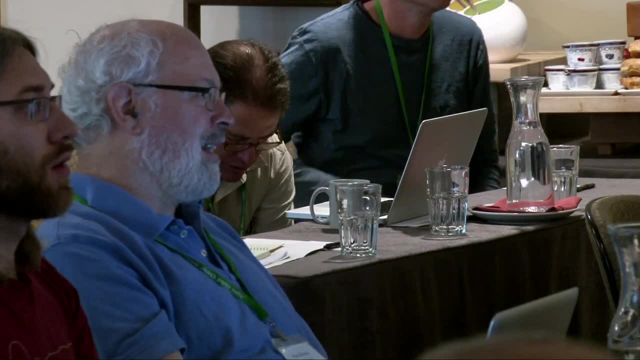 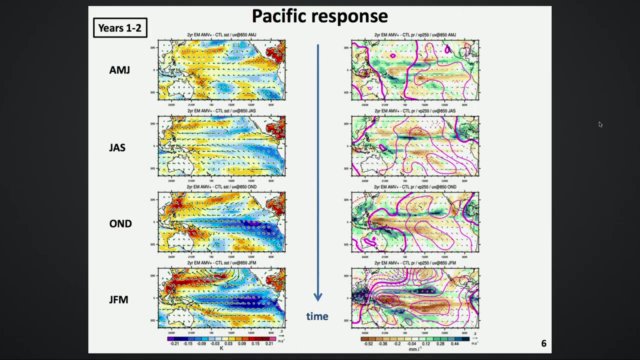 And so I just wondered why you chose that. Yeah, but it's not sensitive to the definition. It's not sensitive to the definition. It was just easier for me to split in three months the year, So that's the only reason I did that. 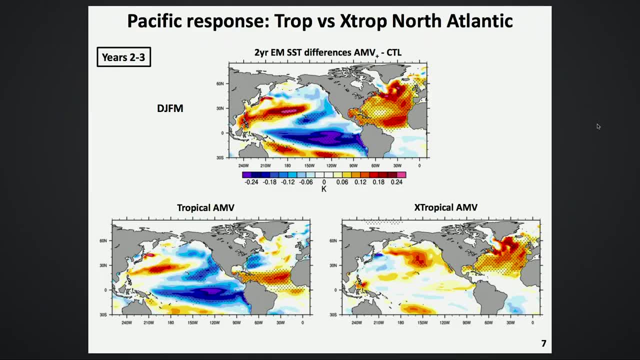 But after I just showed DJFM everywhere. So it's really similar to what I obtained in JFM here. So if you can see here, it's really similar to what I obtained here. And why NEO3 rather than NEO3.4?? 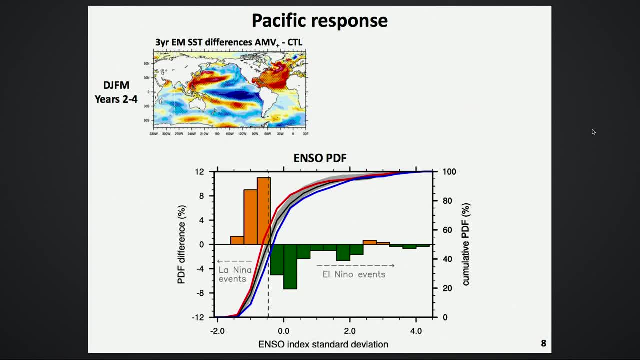 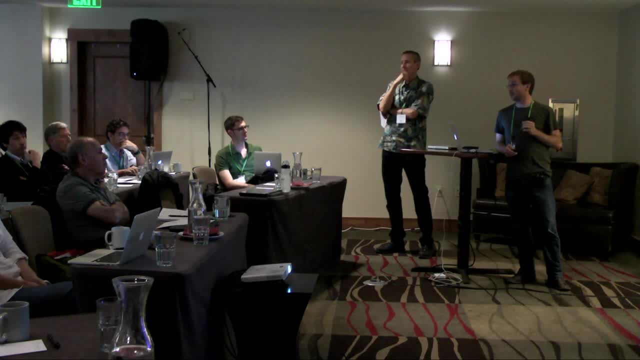 NEO3.4 is because I was just looking at the temperature anomalies And NEO3.4, I think, is a mix between temperature and wind. So I just look at NEO3.. It just adds another segment to NEO3. It goes a bit west. 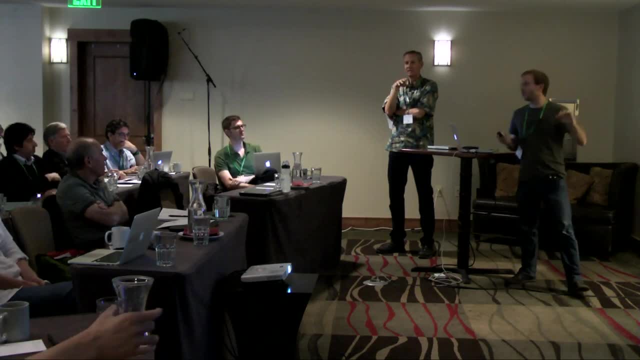 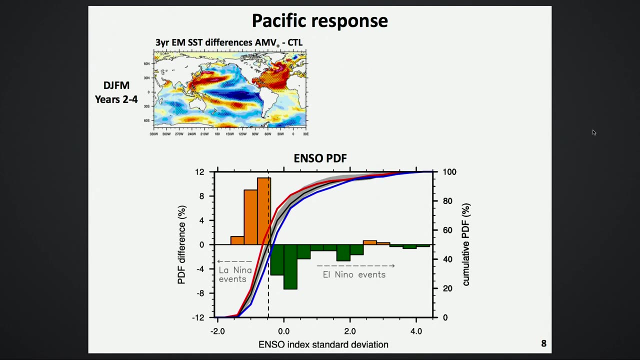 It's not shifted. So yeah, But the thing is here actually. so in this cloud I chose NEO3.. But here it's not NEO3.. It's actually a new action, NEOF, based on the temperature average. 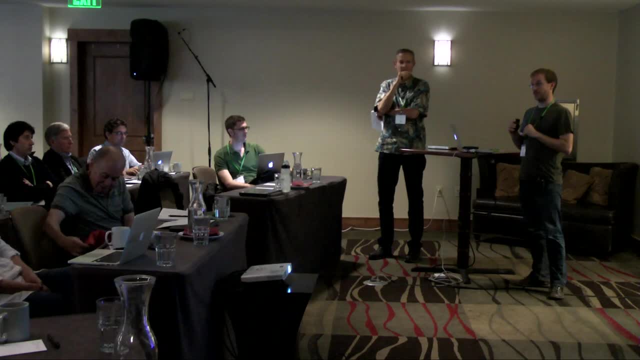 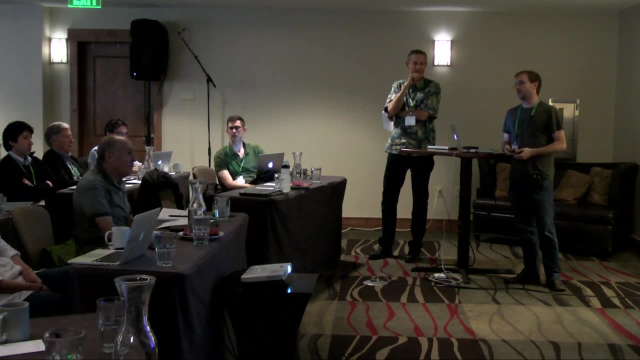 over the first 200 meters of my tropical Pacific And I just completed the first 2F And then I project all my numbers on this 2F. So I mean, yeah, the dynamics is really NSO dynamics, even if I choose NEO3 or NCO3. 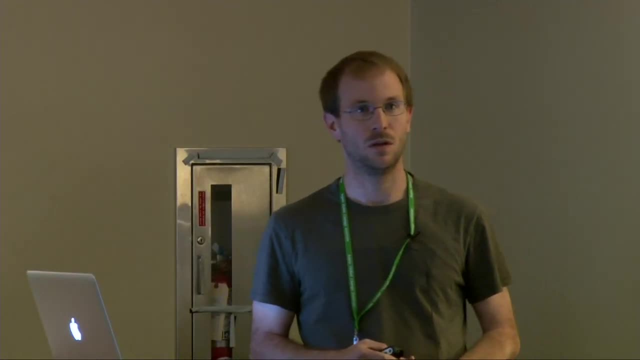 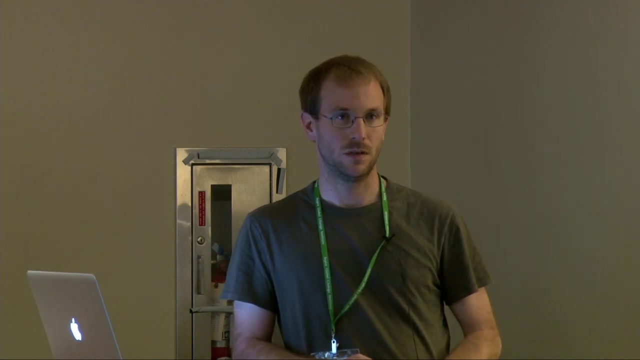 I think it's not sensitive to this. Yeah, so the result is very consistent with our results at Atlantic in this Pacific due to the worker selection. But I'm just wondering in that trend in the Arctic, tropical Atlantic warming is affected there. 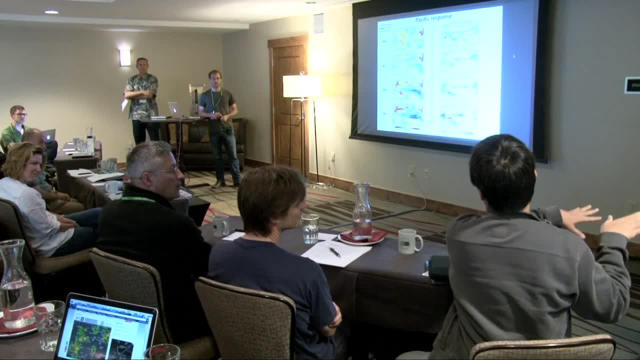 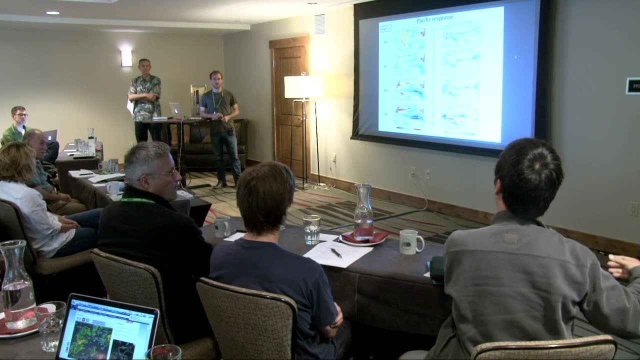 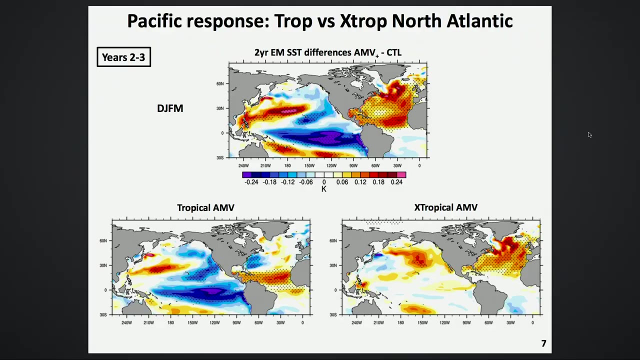 I'm just wondering: is it really tropical Atlantic warming Or is there some gradient in tropical Atlantic is affected with it? In other words, what is the rule in southern tropical Atlantic? it doesn't matter, in conditioned world it's still. Yeah, in this case, we can see the gradient. 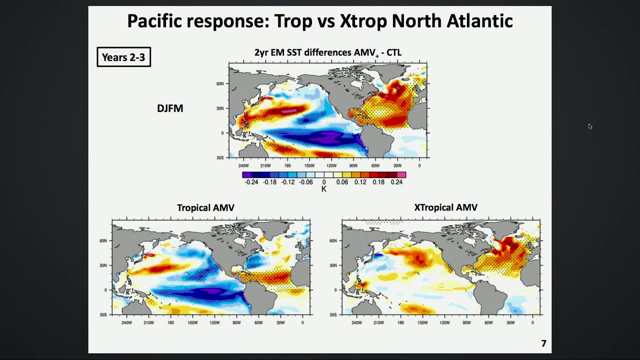 in the tropical Atlantic. So I'm just wondering: If, Yeah, Southern tropical Atlantic is much warmer or colder condition, is there some impact to the Pacific or what's the reason? I don't know. Yeah, I don't know. We can't even know. 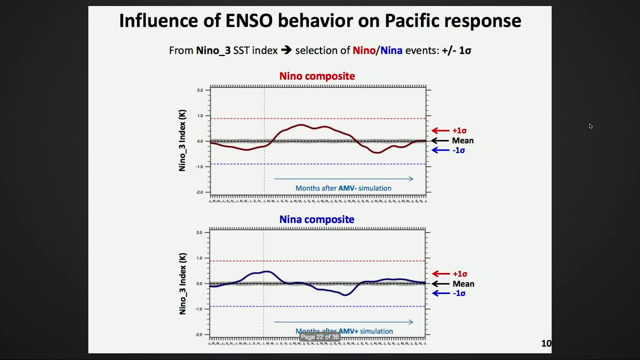 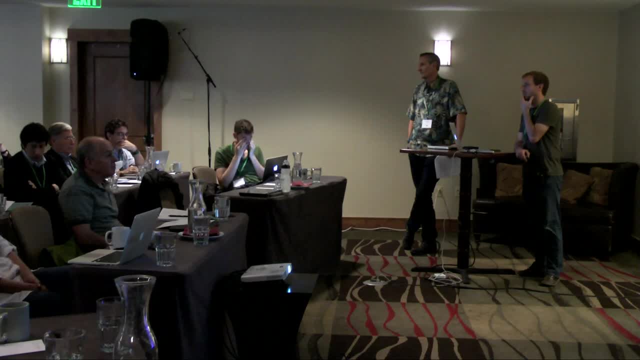 But So I noticed you in this case you don't have, there's no response and also no response, And then negative and there's also no response. So I was wondering if you compare this with the actual models in a couple of models. 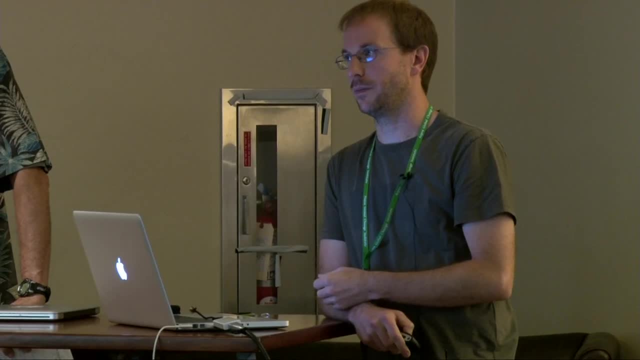 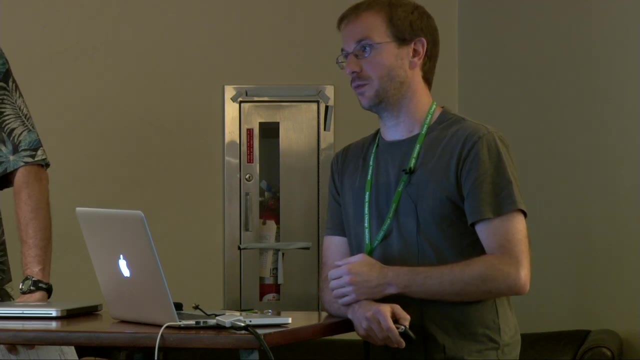 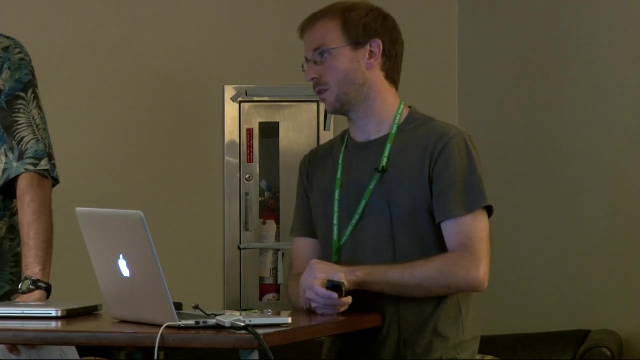 Yeah, I still didn't do that. But, as I said to Gokhan, I think the tropical signature of the model is weaker. So yeah, I have to check. Actually I don't, But I think it could be because your model. 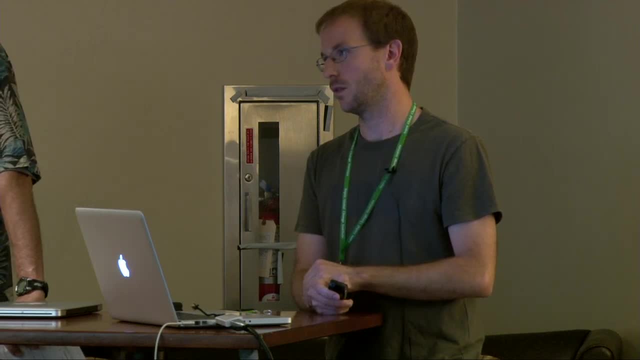 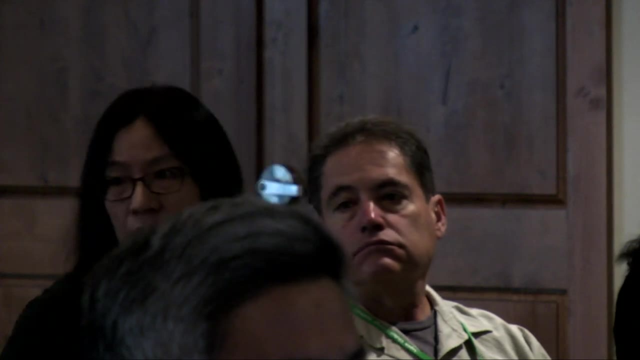 in this kind of setting. your tropical Pacific SST is so strong that could compensate for some of the response to the Atlantic SST. This is what's happening here, But the winter in the end, Oh, it's in the end, OK. 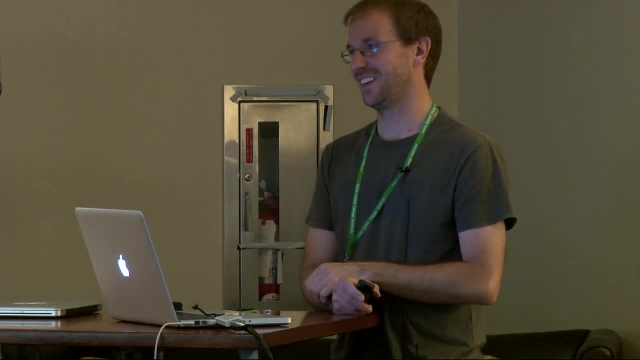 Sorry, I didn't catch your question. No, So this results. I mean you find this on the seasonal times because there's quite a lot of work showing both the equatorial Atlantic SST and the north tropical Atlantic SST and the lead the interseam of about six months or so. 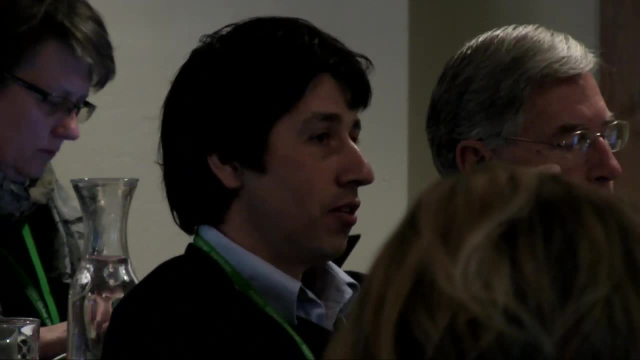 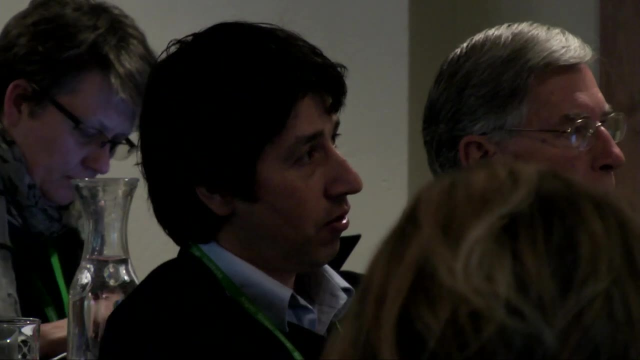 So I think this is very consistent and it's very nice. It seems, if I'm not mistaken, that the response in the Pacific depends on the model having a skewness in ENSO right. Is that true? You must say you have a rectification effect. 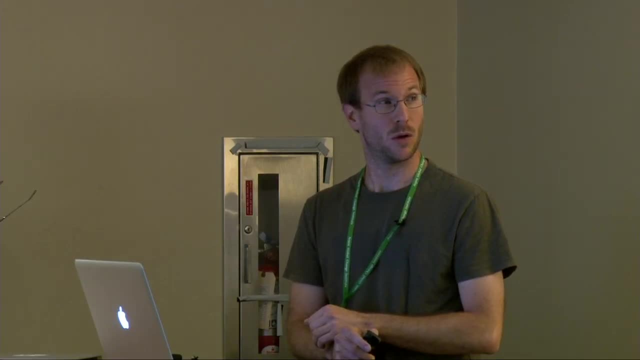 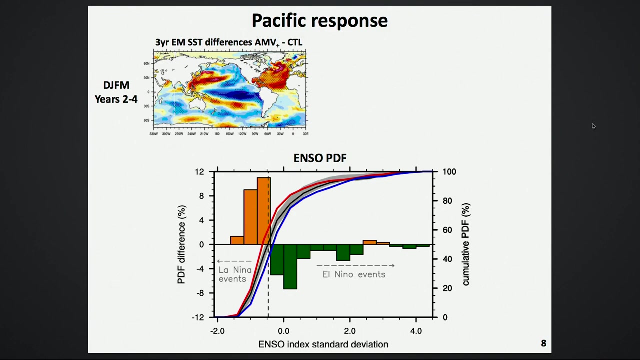 Isn't that what I see? just even on that figure. there There's two lengths of ENSO exhibit. So it's only if you have a positive, if you have a negative in the Atlantic, you will tend to get the positive phase in the Pacific. 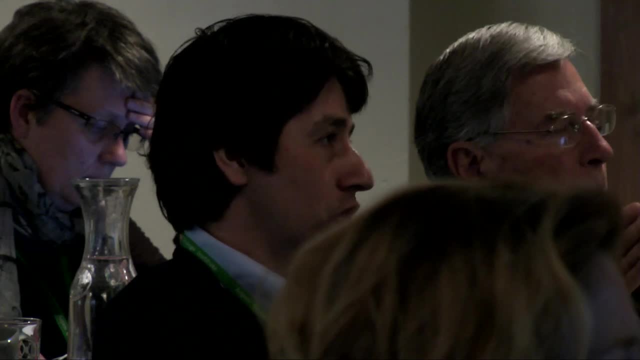 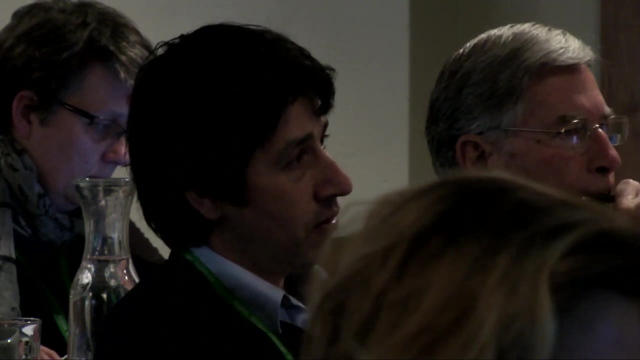 right, Yeah, Right, Yeah, yeah. And the other way, I wouldn't expect such a strong response. if the La Nina is weaker, right, The La Nina's are stronger than La Nina is. Yeah, Yeah, So it's the figure you showed before, right? 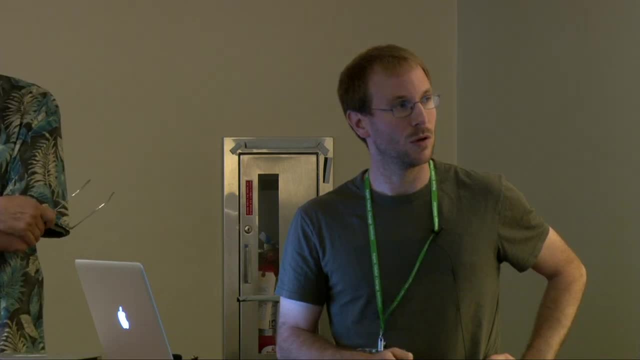 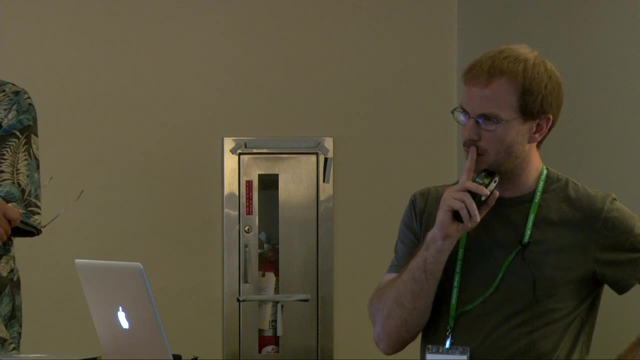 The next two or three. So what do you do, Isn't it? because it takes 10 years and you get one: La Nina and La Nina. La Nina and La Nina dominates, But La Nina's are much stronger than La Nina's. 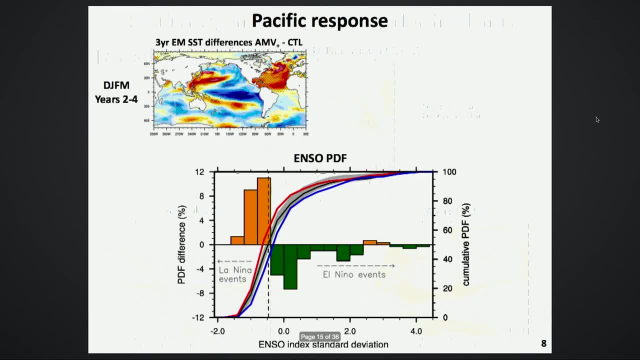 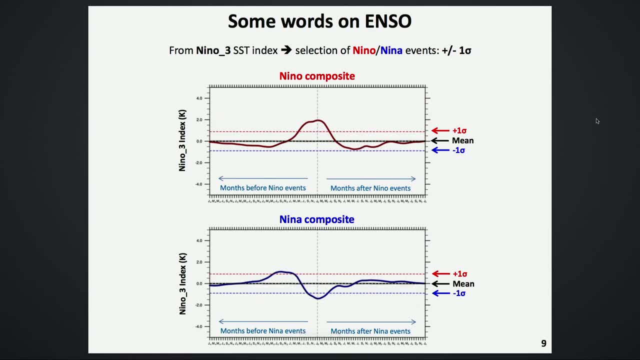 Oh yeah, But actually if you look at the But, if you look at that figure there, the one before that. So if you look at this composite here, Yeah, There is a La Nina event there, but then there is weak. 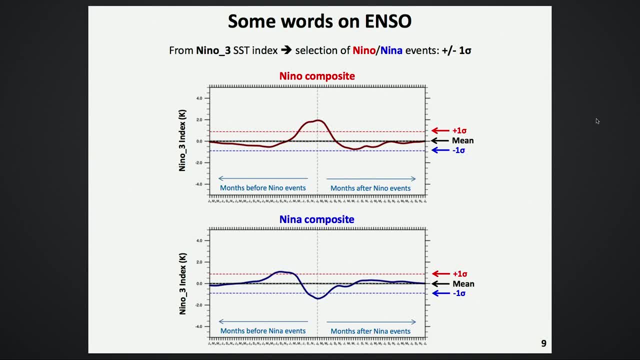 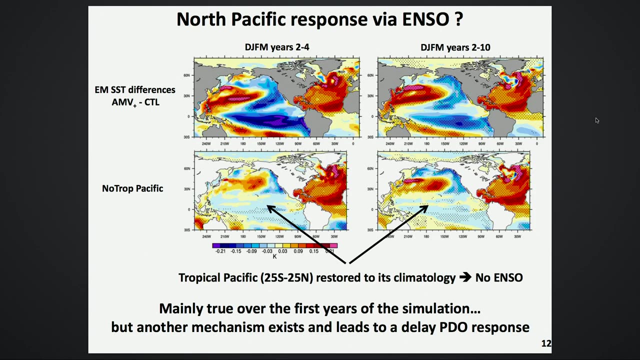 Very weak, Very weak. So that could be a reason why the La Nina event, La Nina anomaly, doesn't dominate the signal. But if you compare this map here and this map here here, it's only an average of the first three years. 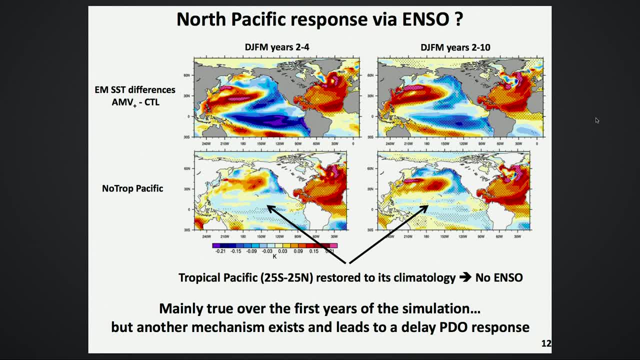 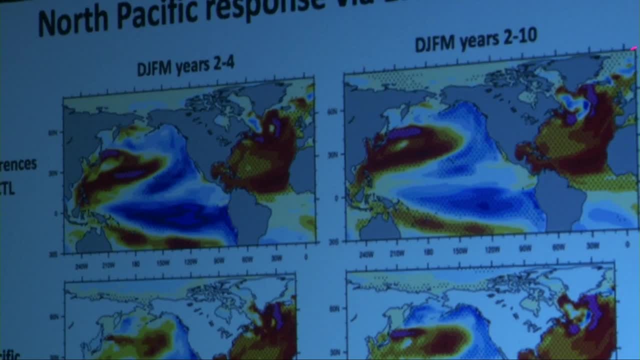 of the simulation. So there is strong cooling here. But when I average over all the 10 years the cooling is much weaker. So it can be due because I've got much more sample, But as well because in this average there was as well Nino events at the